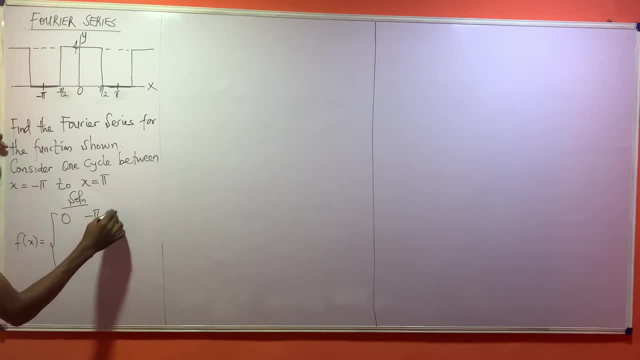 0 at minus pi less than x, less than minus pi over 2.. Yes, this very range for x, So this very range. That's what we have. And what about the next guy After minus pi over 2,? so minus pi over 2,? what was the value of y here? 4.. When s was minus pi over 2, the value for y was: 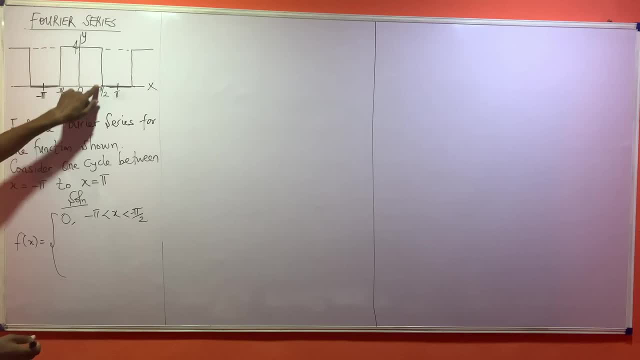 what 4.. Now it continued until what? Pi over 2.. So we then have minus pi over 2 to pi over 2.. And the function value was 4.. So this was minus pi over 2, less than x, less than pi over 2.. That was. 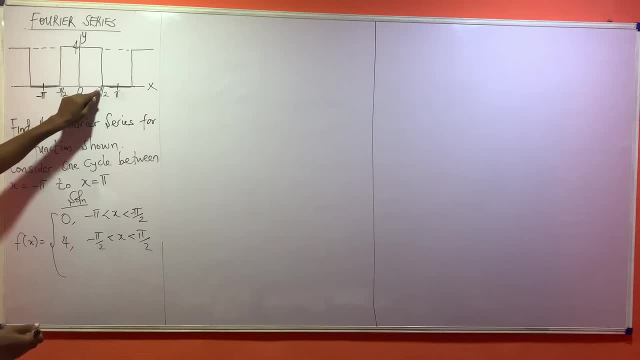 what we had. Now what will be the next thing? again, I have pi over 2 to what? 5, because you said we're going to be ending at pi. So pi over 2 to pi. what is the value for y here? 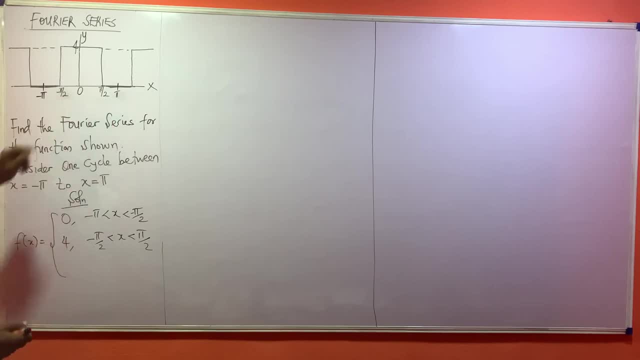 0.. Or you can say: what is the value for f of s: 0. So this will then become 0 at pi over 2, less than x and less than pi. So this is what we have. This is our values, And the next thing I. 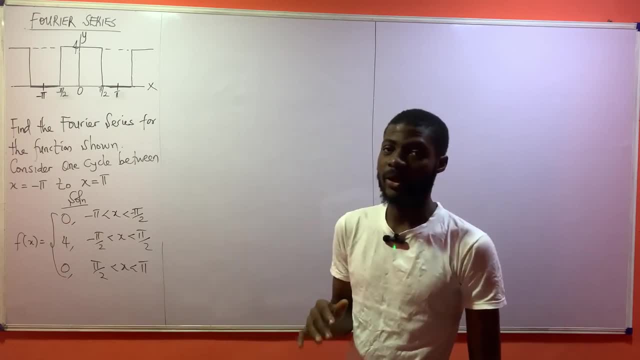 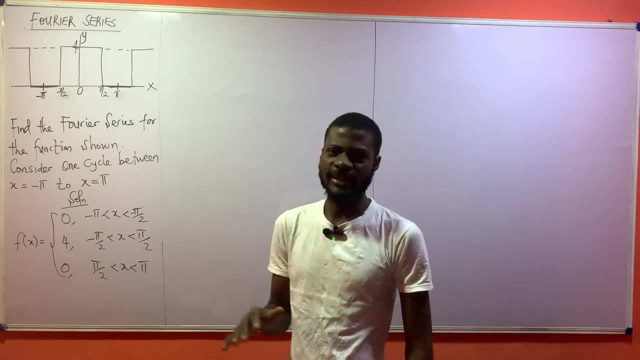 will then do is kind of simple. I will then have to find my coefficients. I'll find my a0,, an and b sub n. So let us get started. These things are very easy, though. They just need us to be very careful. 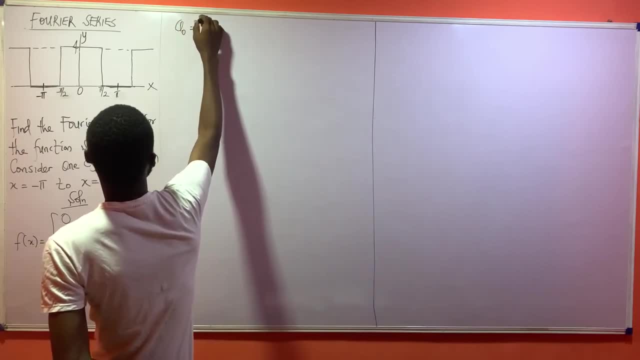 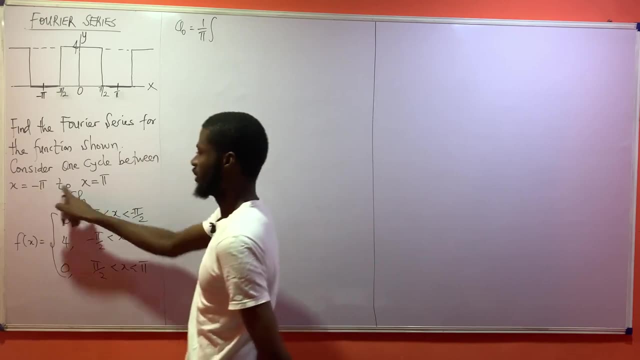 Okay, So what is the formula for a0?? a0 is 1 over pi with the integral from. okay, with the integral from, this is the what's it called The upper and lower limits I'm going to be having. 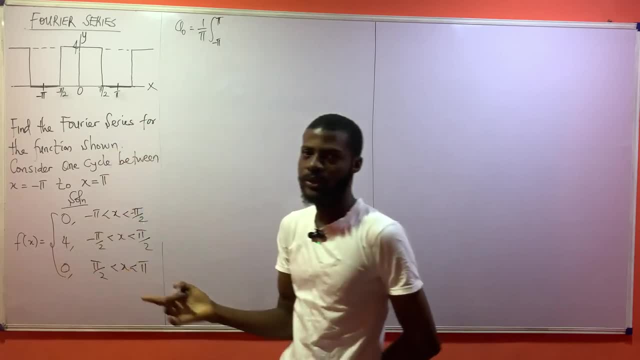 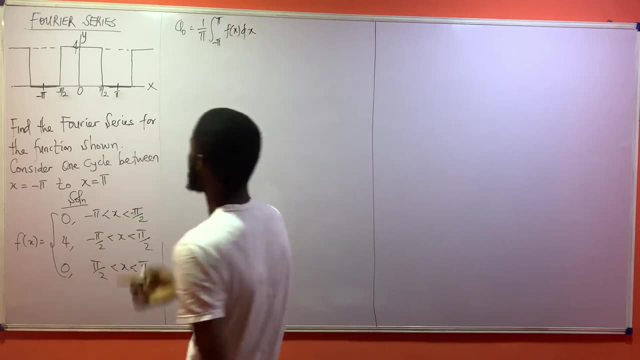 minus pi, So pi. or you can say that as a period. So you are going to integrate over the period. So this will then become f of s? ds. So that's the formula for what a0.. So I'm going to use that formula to solve the question. 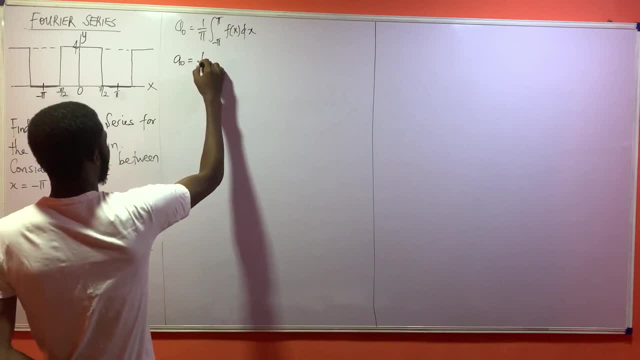 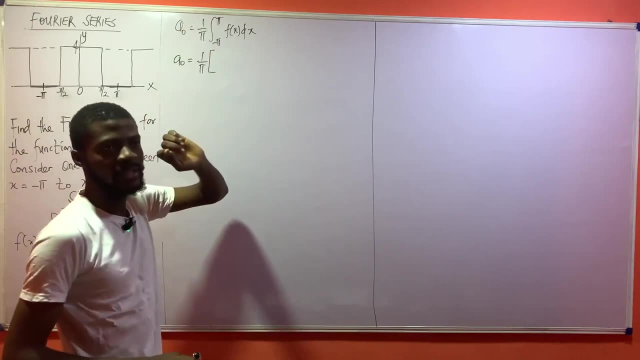 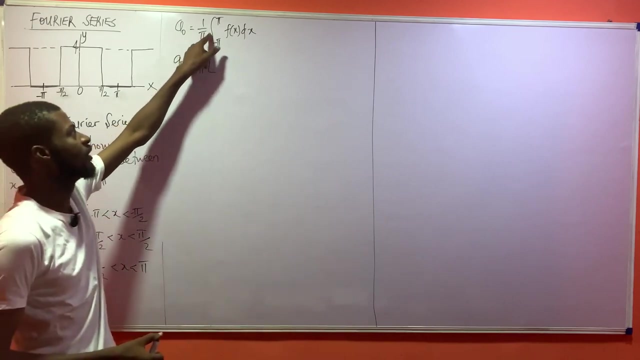 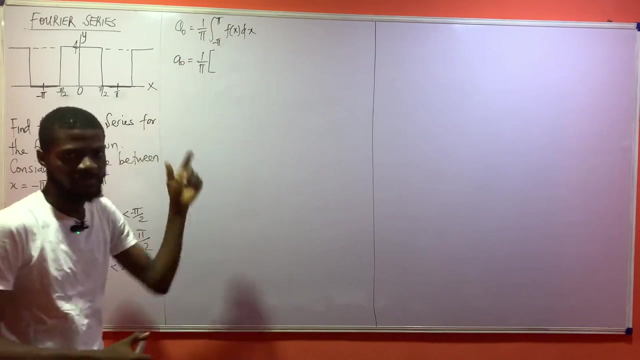 So a0 is equal 1 over pi open bracket. The thing is this: You see, this very integral from minus pi to pi, It's not actually that continuous. It is discontinuous Because for me to solve this very, or rather integrate this very function, there was no f of s value that ran from minus pi to pi. If 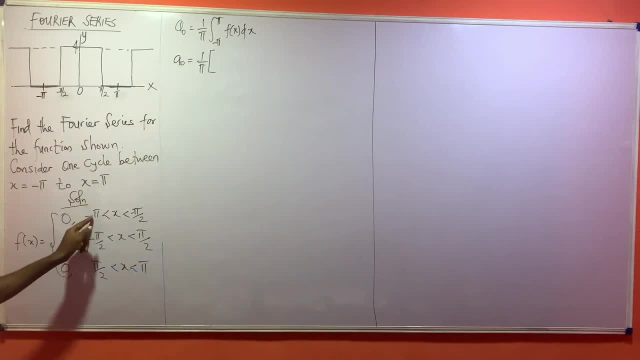 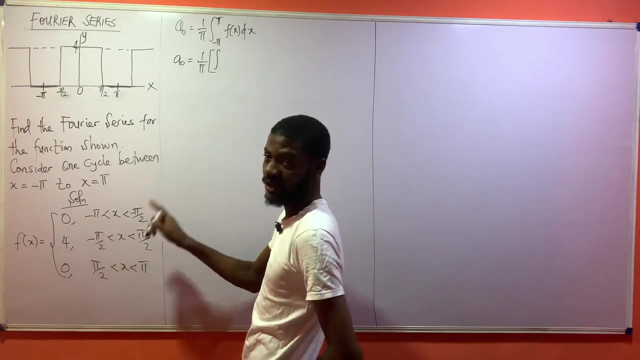 all of these guys? they did not. none of them ran from minus pi straight towards pi. Instead, we had different values for different parts. So it means I can actually express this very guy as the integral from minus pi to minus pi over 2 in the first case. So I'll have minus pi to pi. 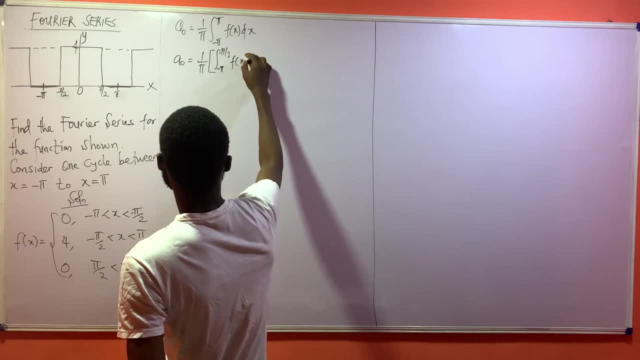 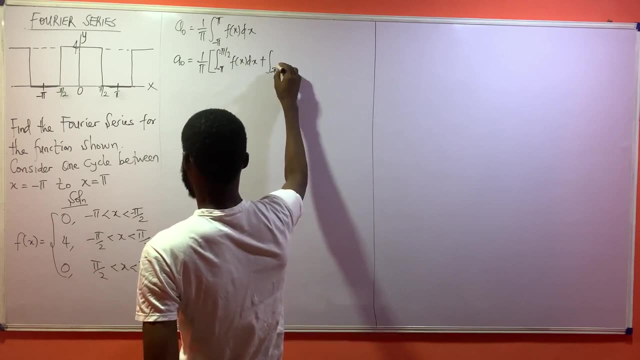 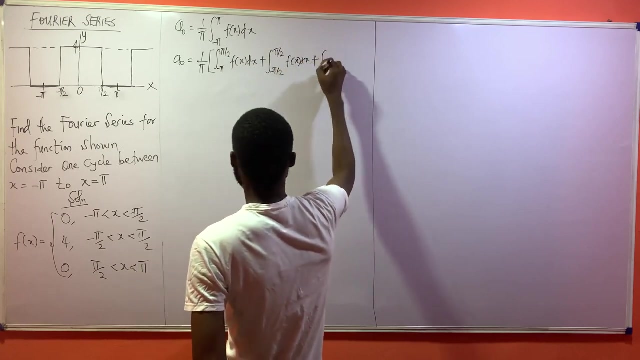 over 2,, sorry, to minus pi over 2, f of s ds plus the next value again: plus pi over 2,, minus pi over 2,, so pi over 2, the input f of s ds then plus. the last one says: 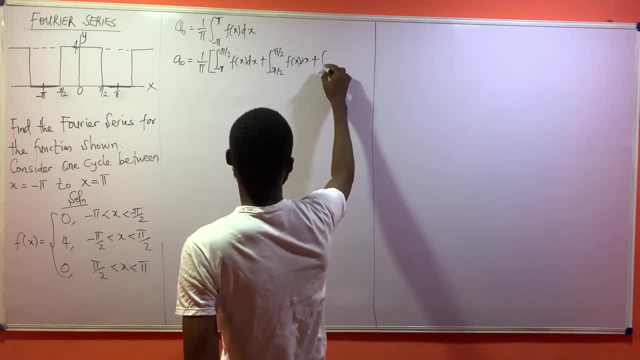 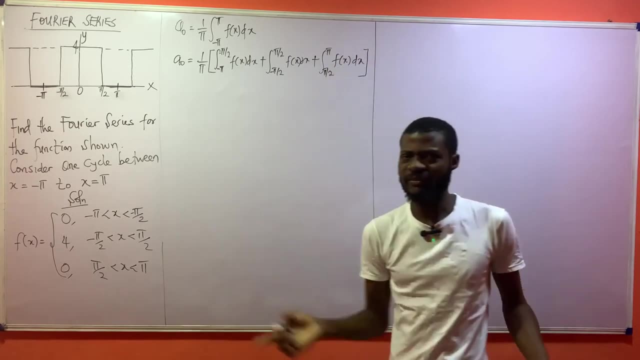 pi over 2 to pi. So this is pi over 2 to pi of f of s ds. So this is all we have. It's very, very simple. You just have to follow the functions that we have So many a times. 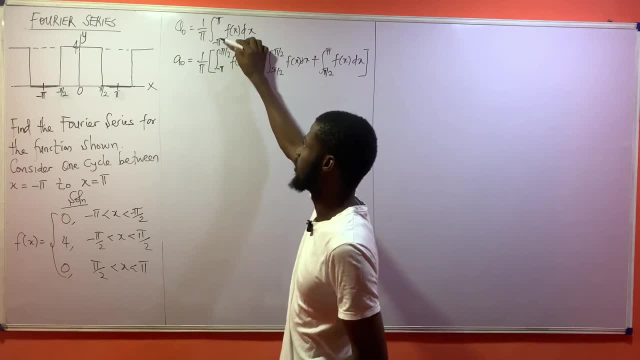 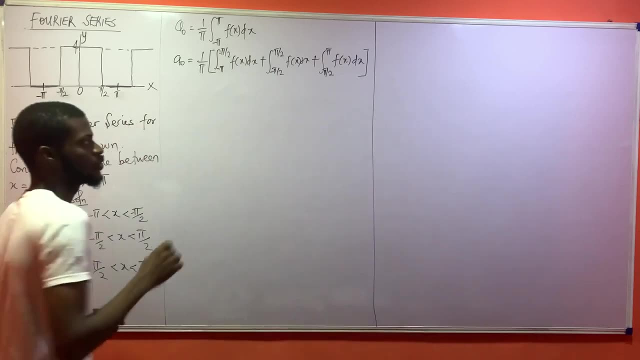 you can just see a particular function value that runs through minus pi to pi straight ahead, But if it doesn't happen, you would have to split the integral. Okay, so this is what we have. The next thing I will then do is to write out these very 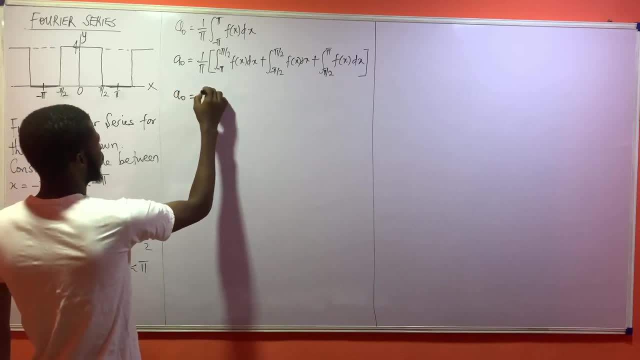 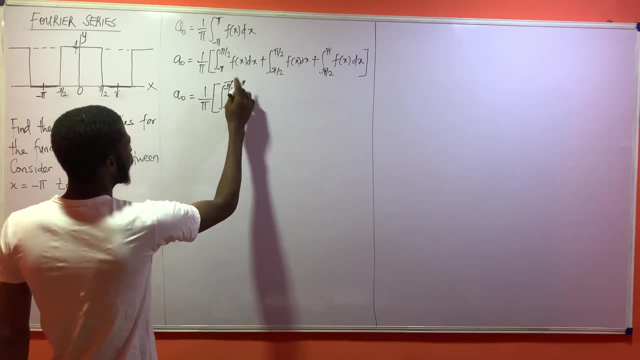 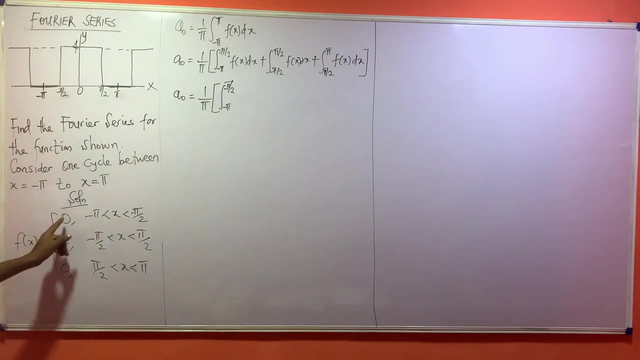 values for f of s. So a naught is equal 1 over pi bracket, integral from negative pi to negative pi over 2.. What is f of s at that very range? f of s is what Equal to 0.. f of s is equal to what? 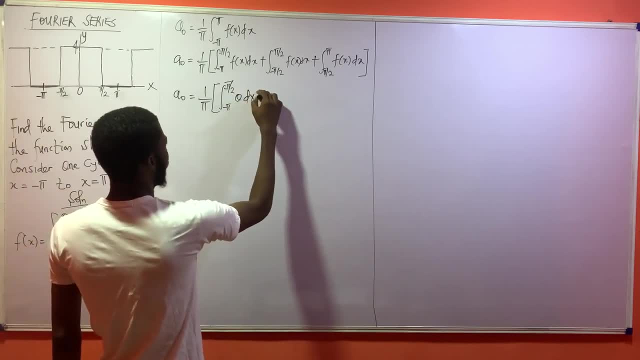 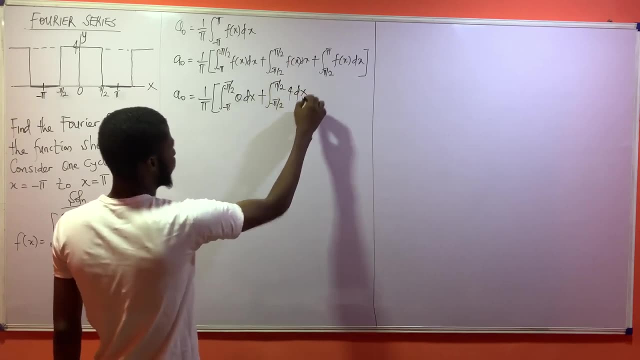 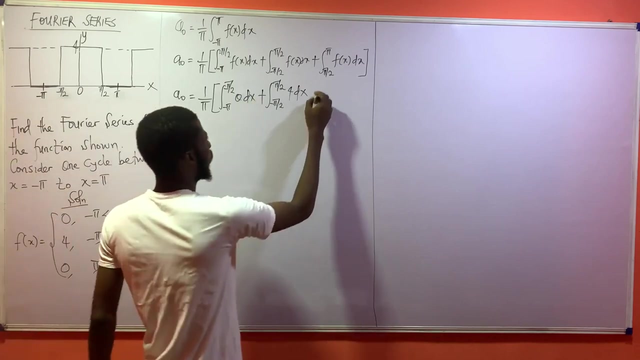 0.. So I'll say that this is 0 dx plus integral from negative pi over 2 to pi over 2.. f of s here is 4.. You put your dx, Look at it here- 4 from minus pi over 2 to pi over 2.. So that's 4.. Then plus. 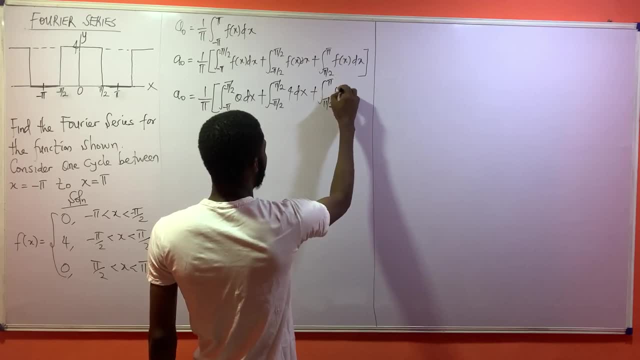 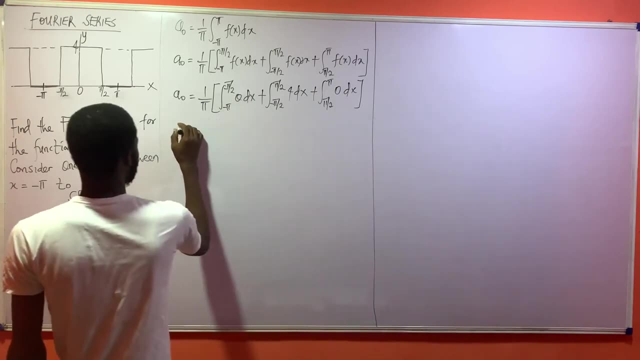 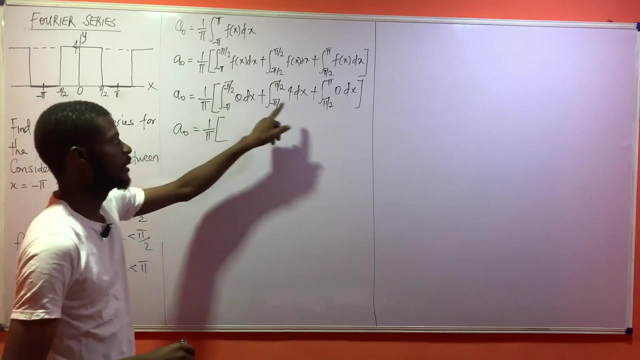 integral from pi over 2 to pi f of s. That is 0 dx. Okay, so this is what we didn't have. This is what we didn't have. So I'll say: a naught, a naught f of s is equal 1 over pi open bracket. The answer for this will give me 0.. The answer for this will: 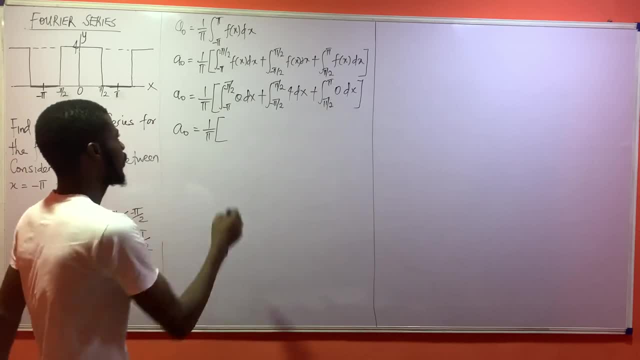 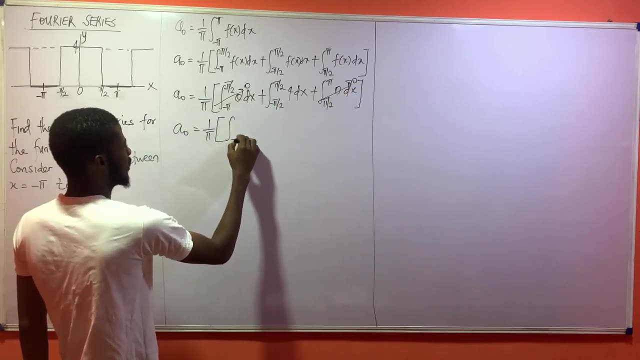 give me what 0. If you integrate 0, your answer is 0.. So everything here is what 0. Everything here is what 0.. So what am I left with The integral from negative pi over 2 and pi over 2? 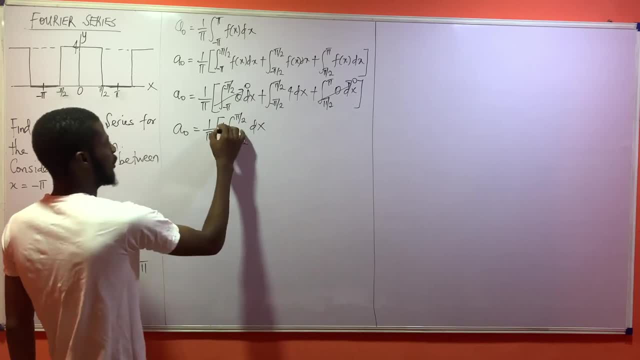 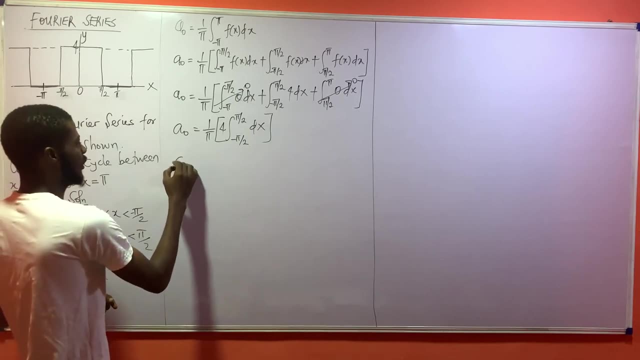 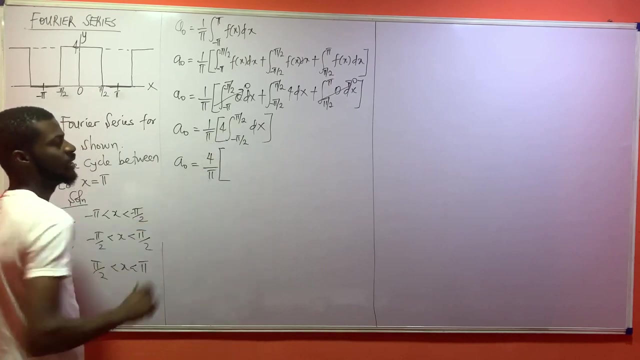 dx. Now this very 4, let me put it here: I can put that very 4 there, because 4 is a constant, 4 is a constant, So I can do that. Now this is a a naught equal 1 times 4, is what 4.. So this is 4 over pi. Then how do we evaluate this very 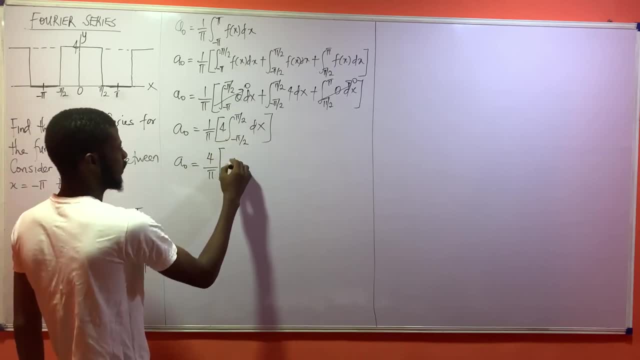 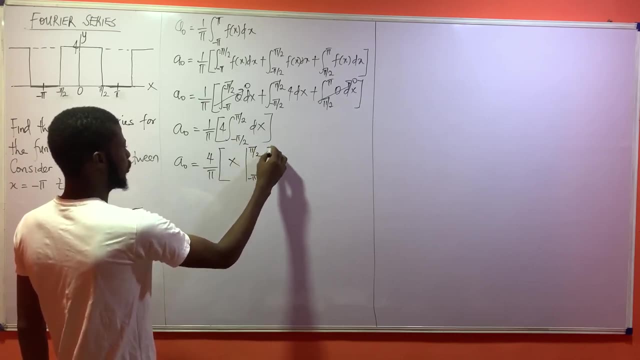 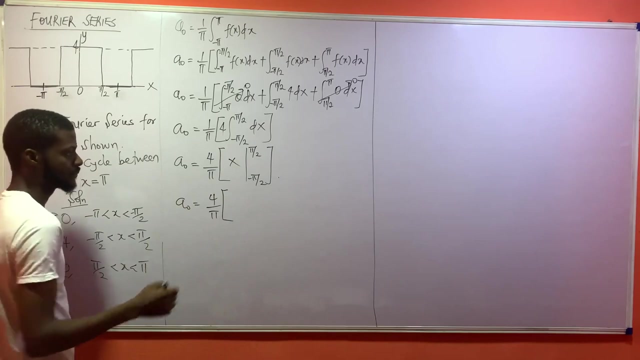 integral. If you integrate dx, your answer will give you x. You put your upper and lower limit negative pi over 2 to pi over 2.. You put this very guy. This will become a naught equal 4 over pi of um. I'll make two brackets this time. In the first bracket s will become pi over 2.. 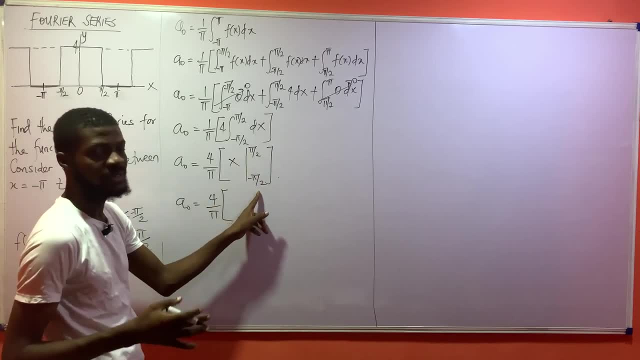 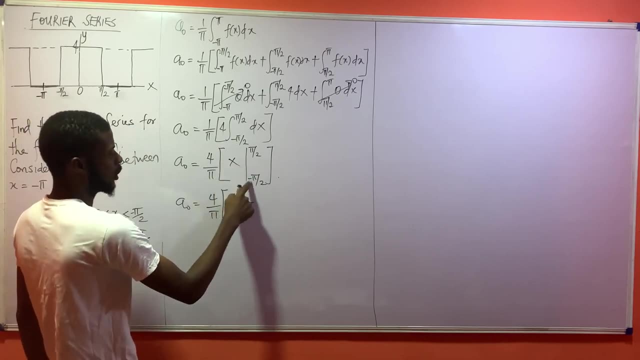 Second bracket s will become minus pi over 2.. Remember the way you evaluate definite integrals. So this will become pi over 2. minus In the second bracket s will become minus pi over 2.. So this is minus pi over 2.. I did not just want to write it. I think it's gonna Okay. 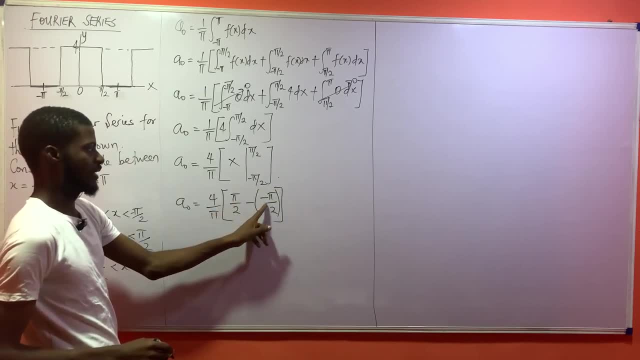 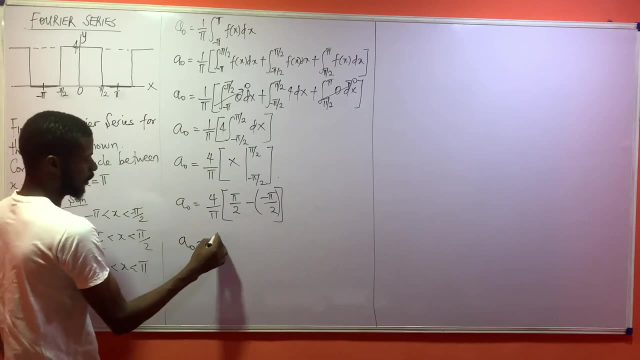 let me just put it So: this is value of x here and value of x here. The first value of s is pi over 2.. Second value for x is minus pi over 2.. So this is a naught equal 4 over pi, Then a bracket. 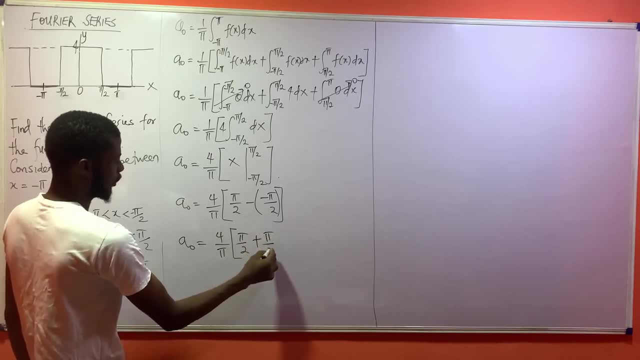 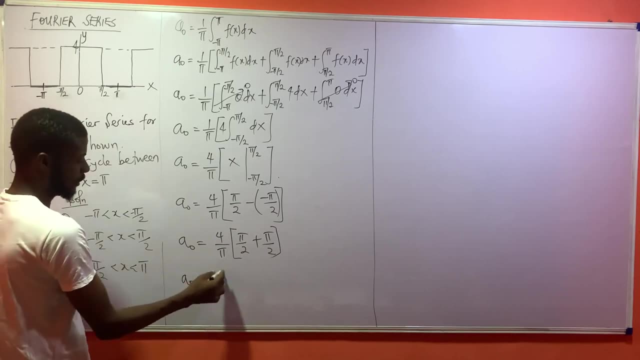 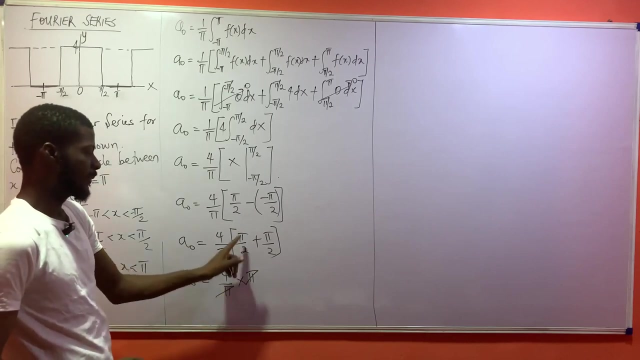 pi over 2 plus pi over 2.. So this is what we have: Pi over 2 plus pi over 2.. So a naught is gonna become 4 over pi times pi. So this we cancel this. Why is it times pi Pi over 2 plus? 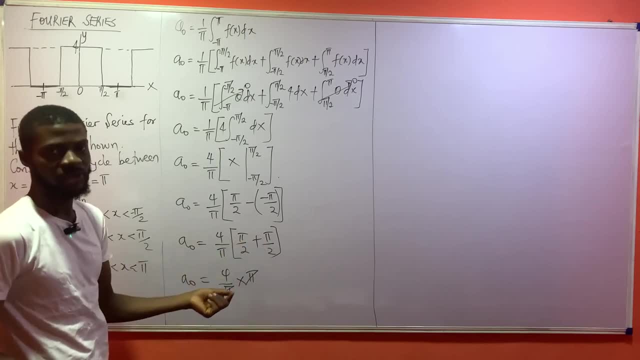 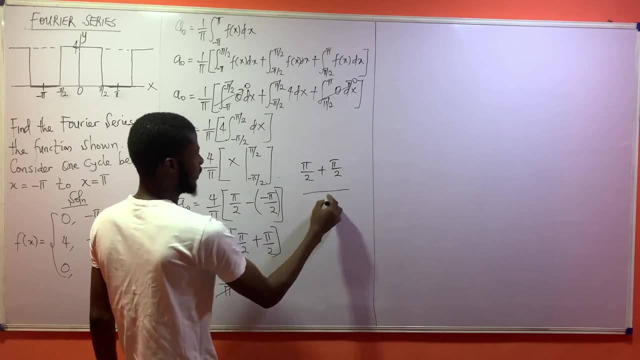 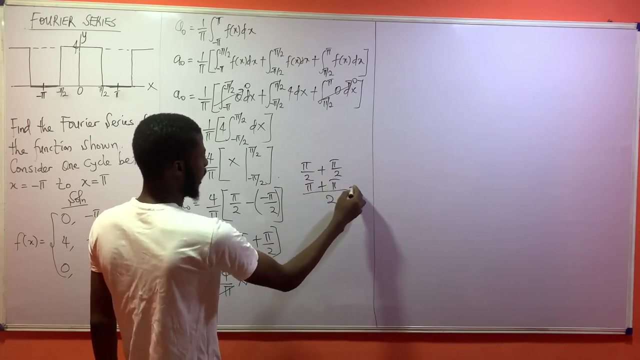 pi over 2 will just give you pi, because they are halves of each other. Or you can do the LCM here. You can say pi over 2 plus pi over 2.. LCM here is 2.. 2 into 2 is 1 times pi is pi plus 2 into 2 is 1 times pi is pi. Pi plus pi is 2 pi divided by 2.. 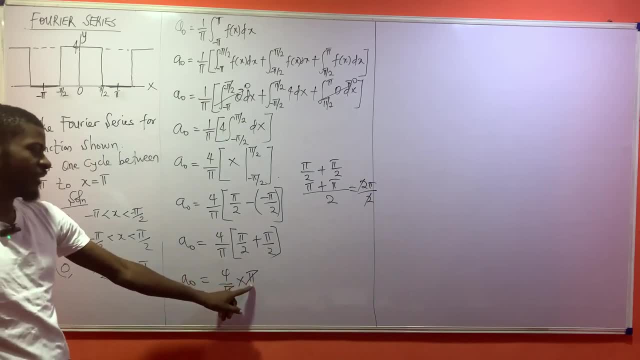 So this will take away this, So that's why pi is left And that very pi can cancel the guy outside. So a naught is equal to what? 4.. Now let me put this answer somewhere: A naught is equal to 4. 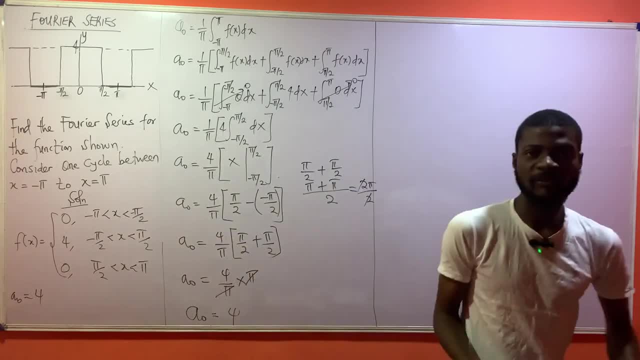 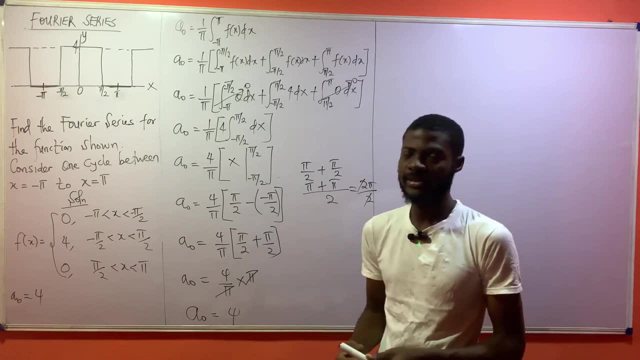 because I may write this part very soon. So that's the value for a naught. Now, what will then become the value for a? You have to take your time. You have to take your time to do all of these things. So what is a sub n? 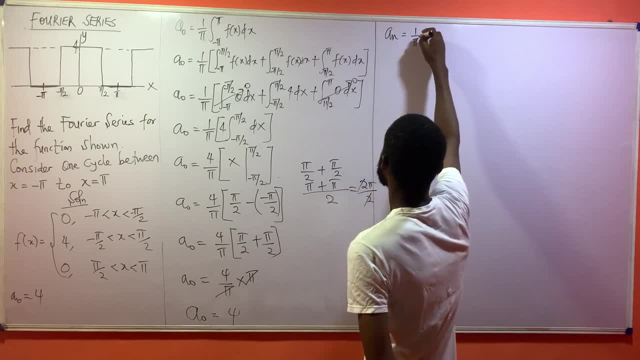 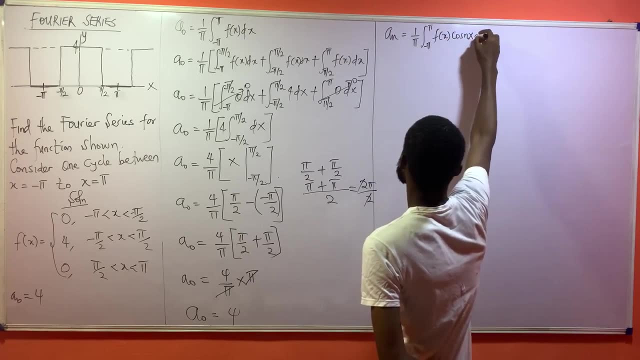 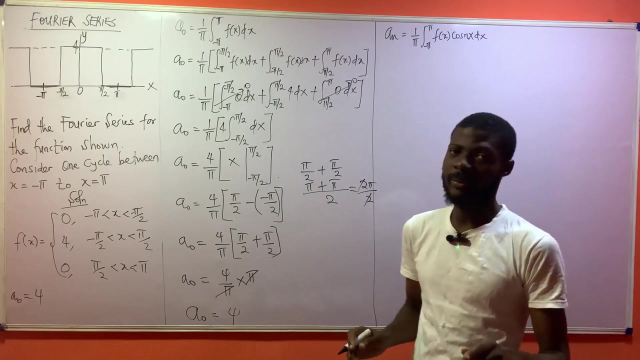 a sub n is equal 1 over pi, integral from minus pi to pi of f of s, cos, nx, dx. So that's the formula for what a sub n. Very simple. Now remember to hit the subscribe button, like this very video. 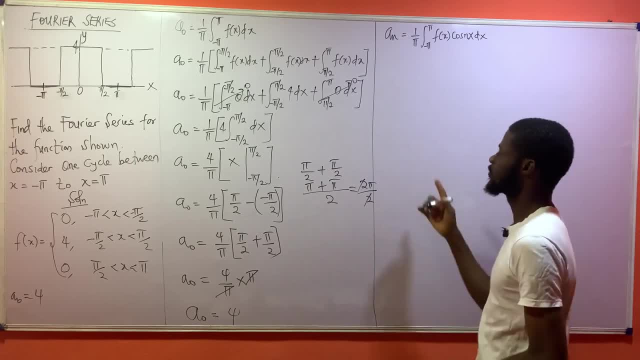 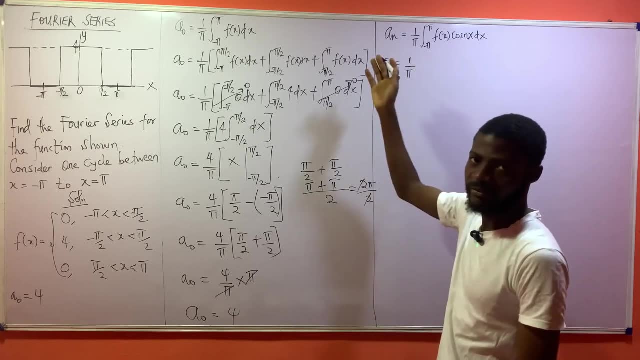 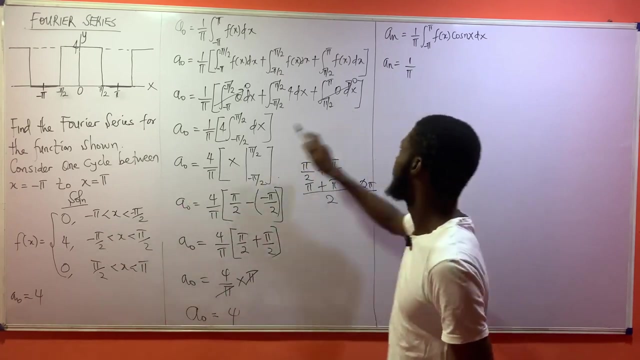 and share it to your classmates. So right now, let us proceed with this. Now, this is a sub n equal 1 over pi. Now you have to be very careful to make sure you can't really integrate these very guys straight, because there was no function value that ran from minus pi. 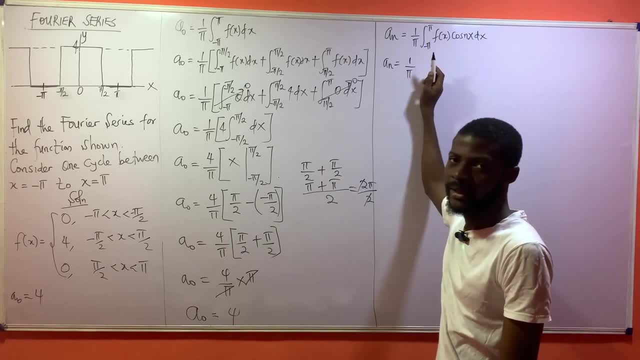 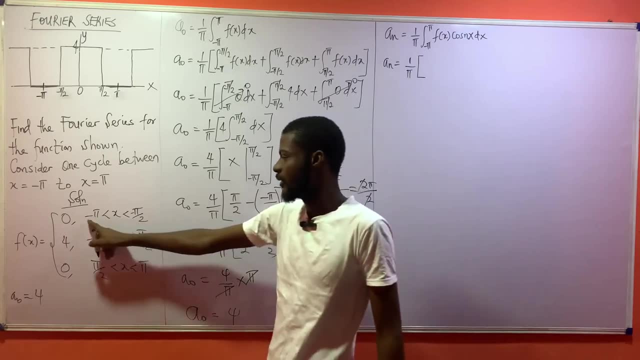 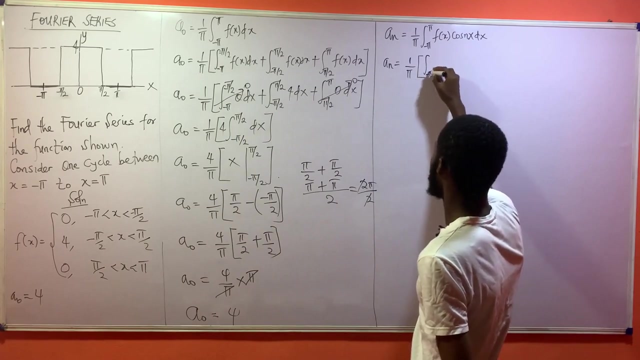 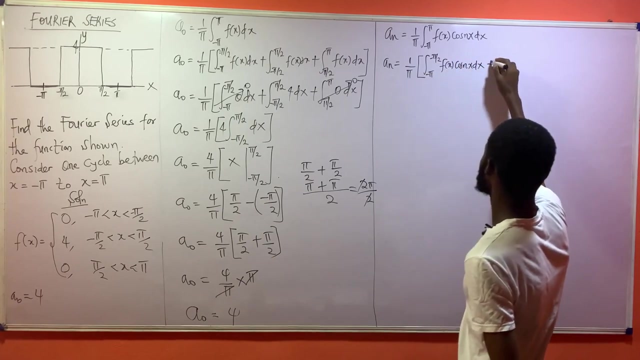 towards pi. No value for y actually ran with this very interval of x, So I'm going to split it down to what we have. We have minus pi to minus pi over 2.. Same thing we repeated at this very part. So we have minus pi to minus pi over 2, plus integral. from minus pi to minus pi over 2. f of s, cos, nx, dx plus. 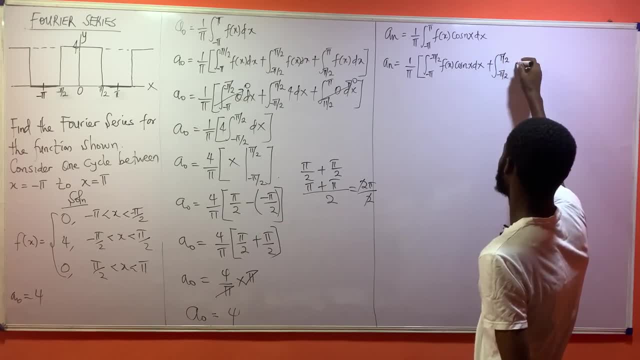 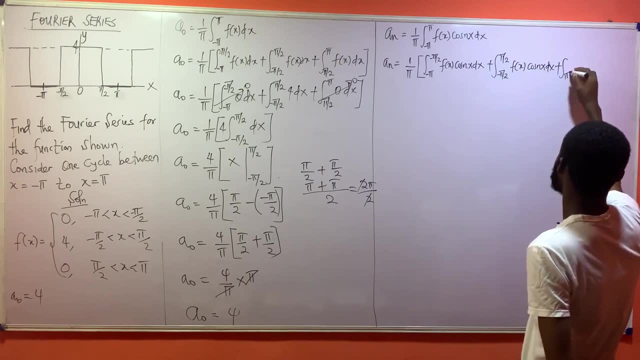 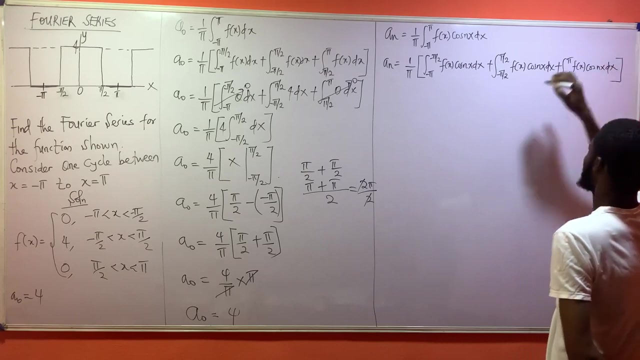 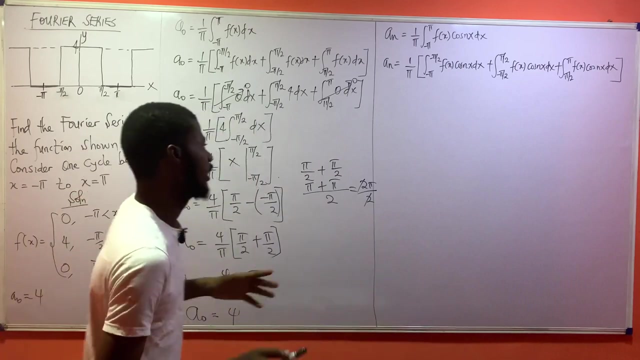 integral from minus pi over 2 to pi over 2 f of s cos nx dx, plus integral from pi over 2 to pi f of s cos nx dx. This is what we'll then be having. Now, if you look at this, you can actually easily solve what you need. Look at this. If this part is, 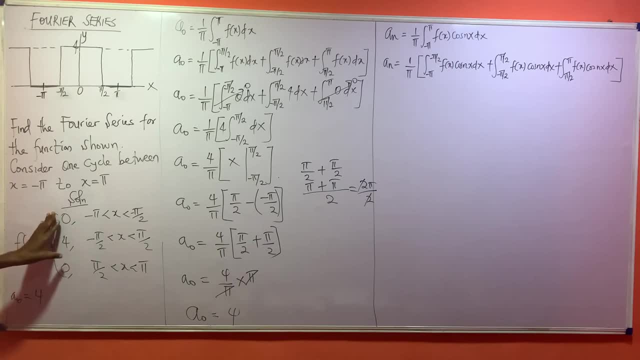 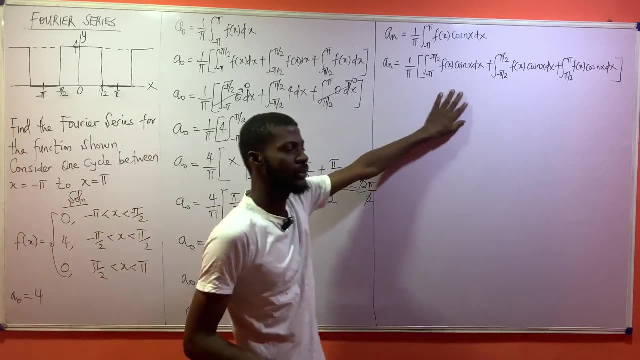 zero and this part is zero. I really do not have to bother about the integration, because my result is going to be giving me zero at the end of the day. So same thing is going to happen here Again. same thing will happen at this very part. f of s value here is zero, So everything will become. 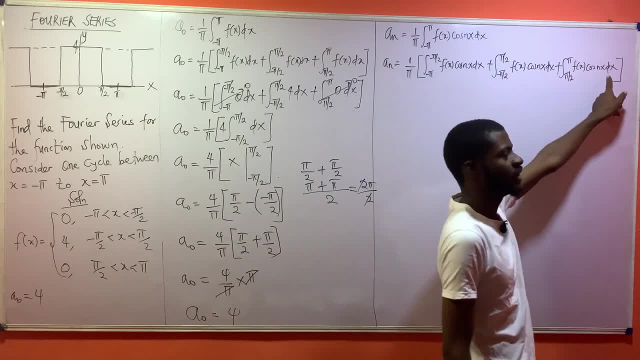 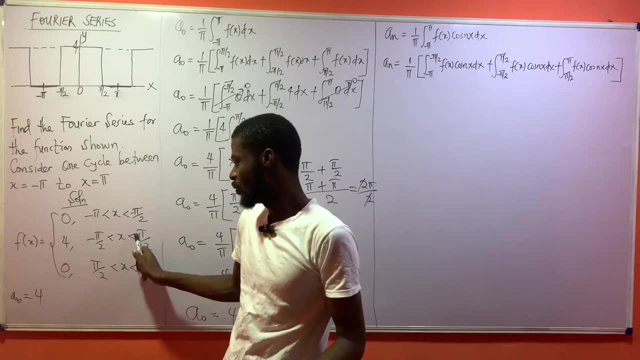 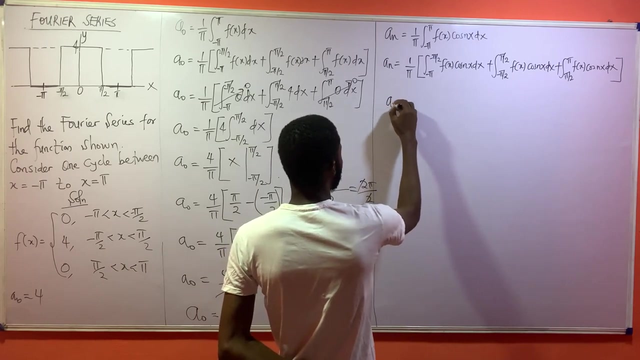 zero f of s value at this very range will still become zero. So the only useful guy I have is the integral from minus pi over 2 to pi over 2, which is the guy in the middle. So you can just easily make everything shorter And you say: this is a n equal 1 over pi. then integral from minus pi over. 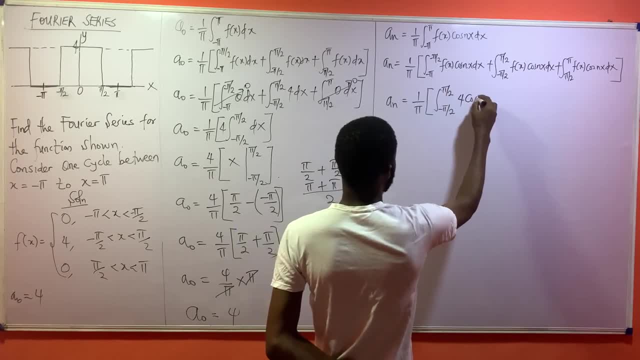 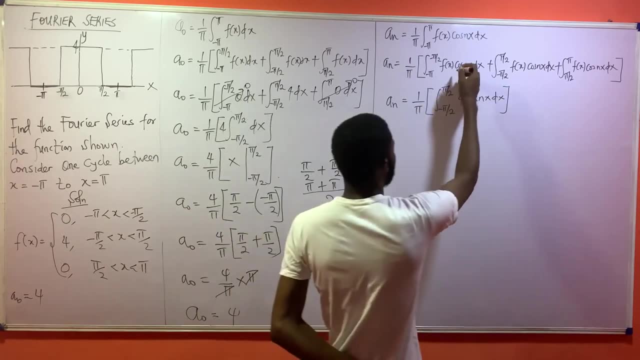 2 to pi over 2 of 4 cos, nx, dx. As easy as that. I believe you know the reason why I just removed all of these guys. The answer here will give me zero. The answer here will give me zero, So don't. 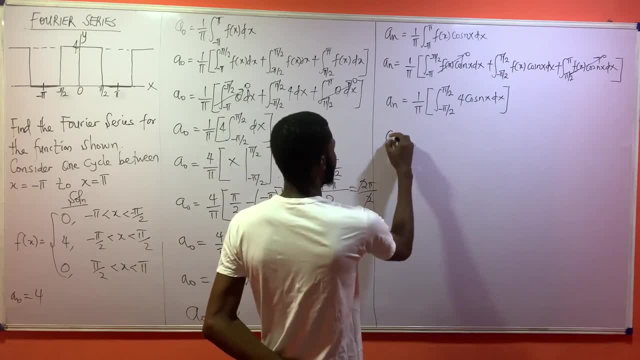 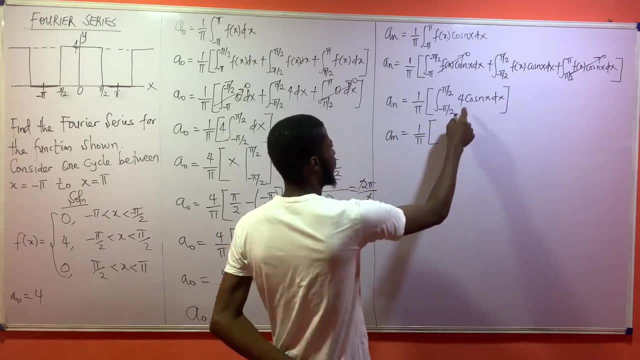 need for us to start writing it again. Okay, Now this a sub n equal 1 over pi. then if you will notice here I love writing it like this- This very 4 can come outside. Yeah, that's true, This. 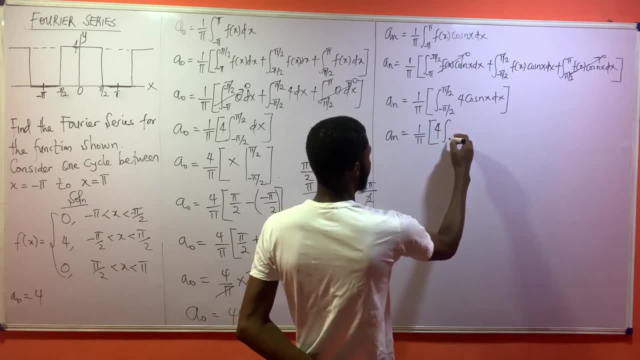 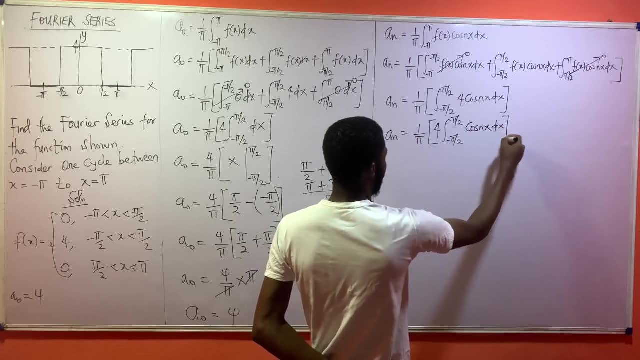 very 4 guy can come outside. So this is 4 integral from minus pi over 2 to pi over 2 of cos nx, dx. Now I can do that. Now what will be the next thing that I can do? I will say that this is a sub n. 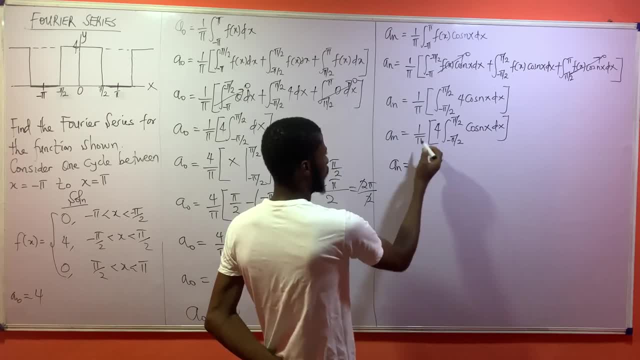 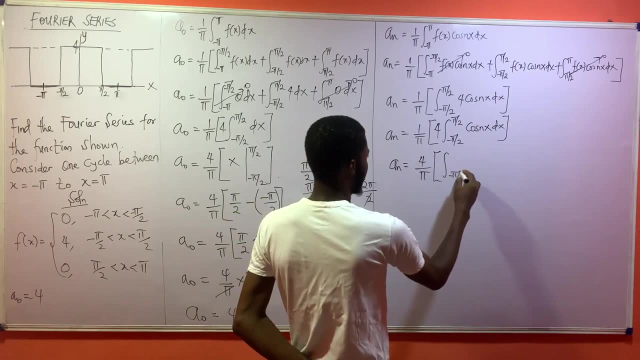 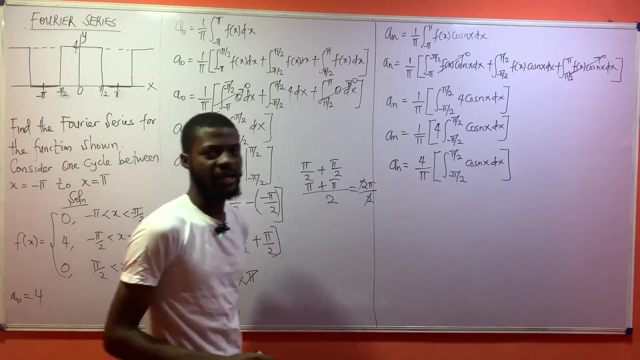 equal 4 over pi. 1 times 4 will give me 4.. So that's 4 over pi. Then I will be having the integral from minus pi over 2 to pi over 2 of cos, nx, dx. So this is what I'll be having left. 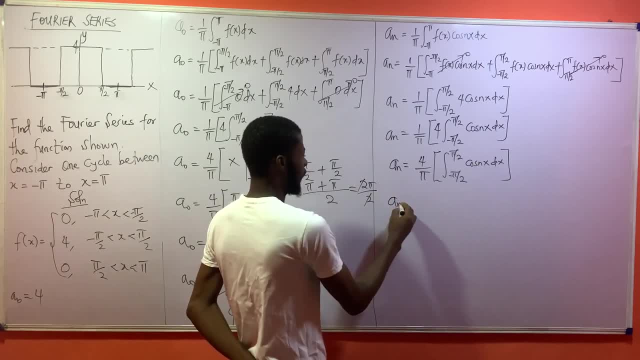 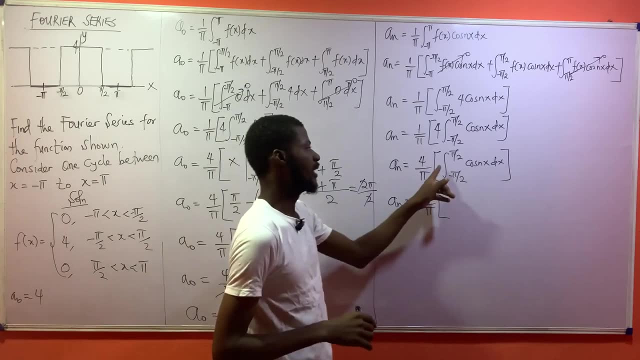 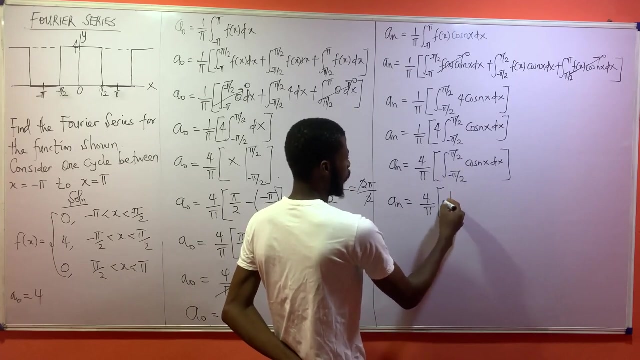 That guy will be left. So let us proceed. a sub n will become 4 over pi. Then, if you look at this bracket, if you look at it carefully, how do we integrate cos nx? First of all, differentiate nx. What will we have? n right? So I'm going to say 1 over n. 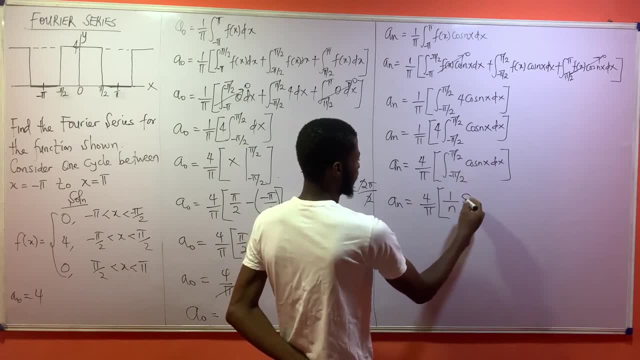 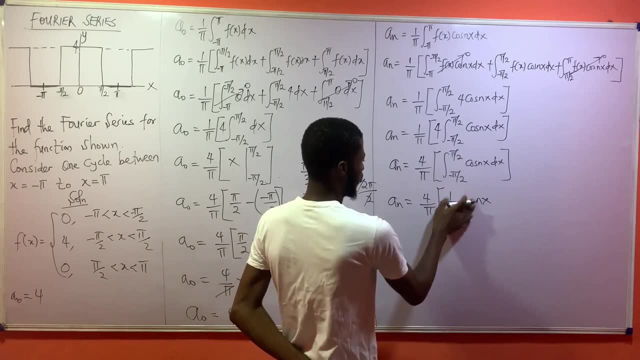 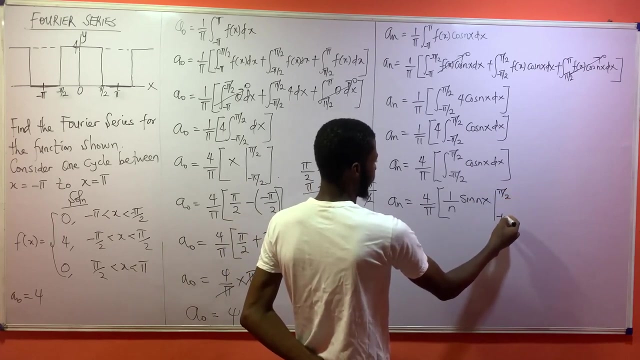 1 over n. Integrate cos. What will you get? Sine You put back that angle nx, So this will become sine nx, So this will become sine nx. Then you put your upper and lower limit, pi over 2, to minus pi over 2.. I was supposed to say like the bottom first. 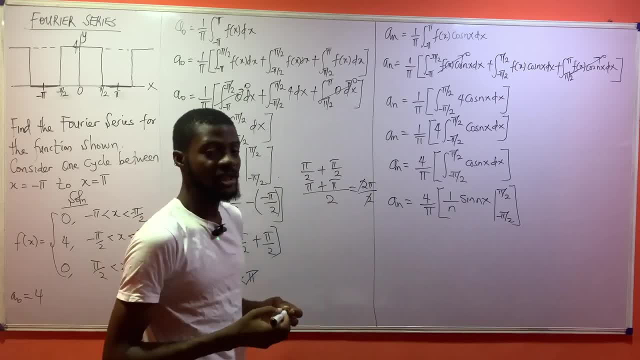 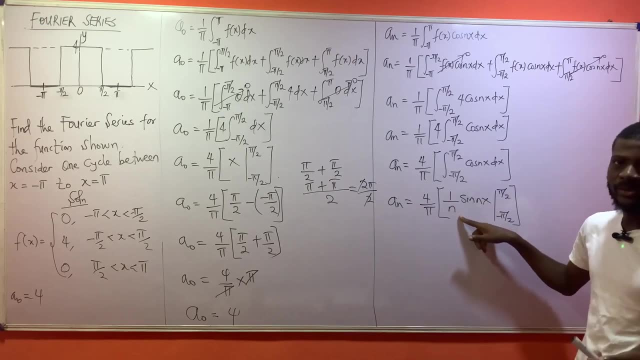 Okay, Now let us proceed with this. If you look at this very guy carefully, carefully, 1 over n is a constant. 1 over n is a constant. So you can actually come outside and I'll say: this is a sub n equal 4 over n pi. I can do it like this: 4 times 1 is 4.. Pi times n is what. 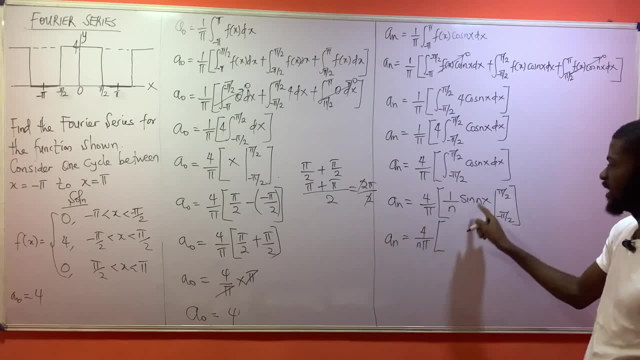 n pi. I can do that. So what will then be left? inside this very bracket I'll be having sine nx, from minus pi over 2 to pi over 2.. So this is what I'll be having Now. this: a sub n equal 4 over. 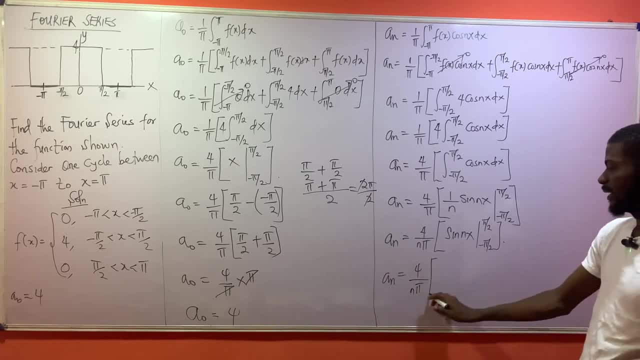 n pi, this very guy which I have. Then let us evaluate this. How do we do it? Remember, we're going to have two brackets. So in the first bracket, anyway I see x because it's dx, Anyway I see x, it becomes pi over 2.. Then what if I see x in the second bracket, it becomes minus pi over 2.. 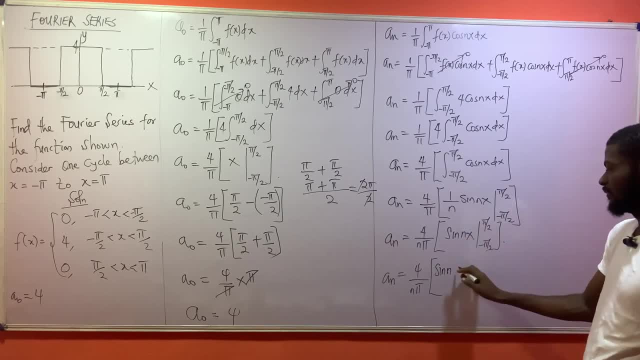 n. Then this s is what Pi over 2.. So s is pi over 2.. Then, minus The second bracket, this time will become sine n times minus pi over 2.. Yeah, Inside a bracket like this, Yeah, I can do that. 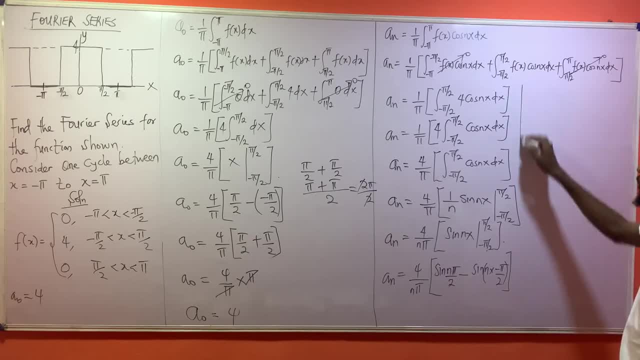 I can do that. Can I come here? Yes, Let me see if I can minimize this space and use this very part. Let me see if I can do that. So a sub n will then become 4.. 4 over n pi open bracket sine n pi over 2. 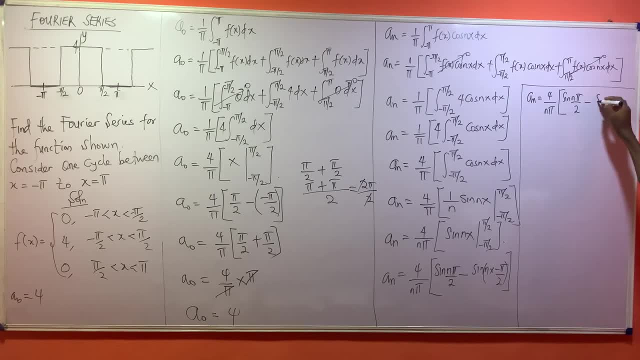 minus sine, minus n pi over 2.. Now look at what I just did here. See what I just did here. I wrote everything, but at this very part I said: n times minus pi will give us minus n pi divided by 2.. That's what we have Now. let us proceed with this. Let us proceed with this very guy. 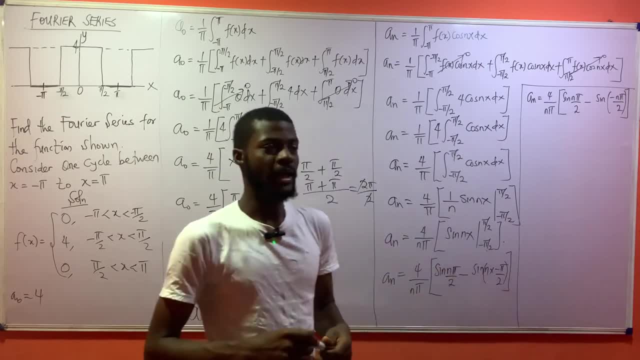 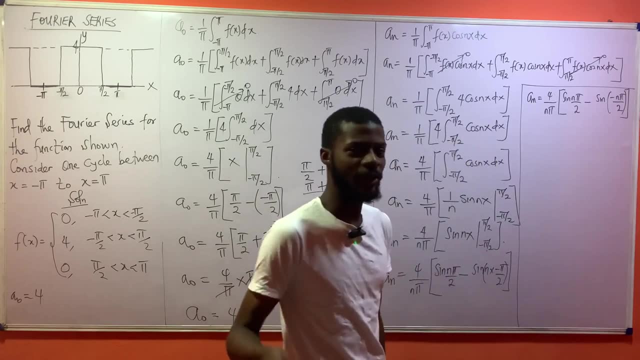 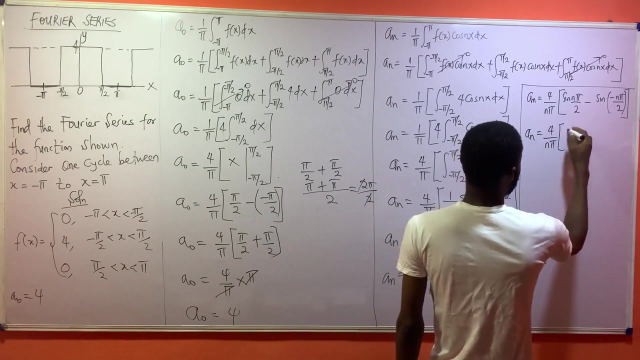 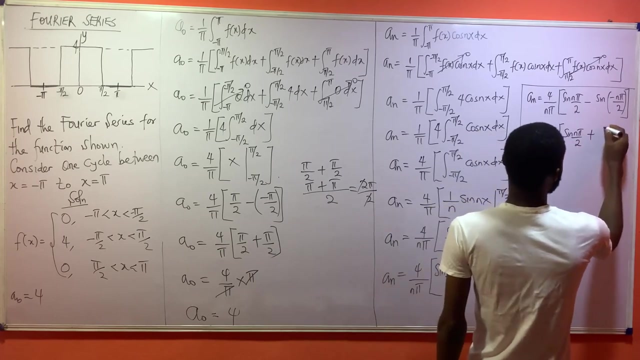 I believe, If you're understanding, please you can comment and tell me what you think You know you can actually discuss with me. I would reply or comment So this: a sub n equal 4 over n pi bracket sine n pi over 2.. Then this becomes plus sine n pi over 2.. Okay, Why did I say plus? 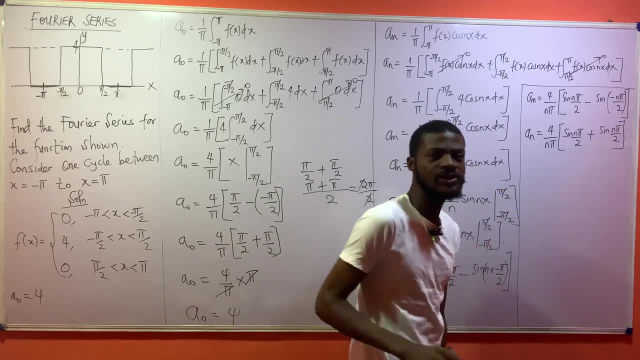 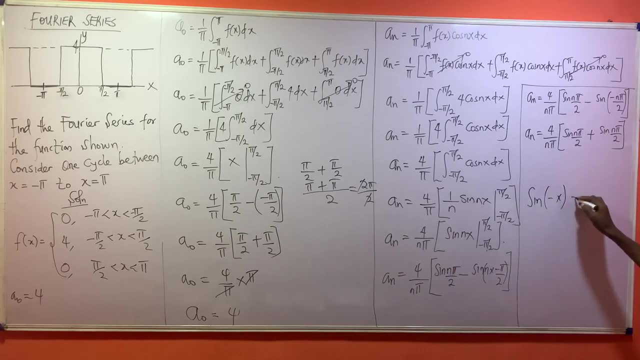 Why did I say plus at this very side? Now please remember that in signs for all signs, sine minus x is equal minus sine x. Yeah, This minus sign can come outside, The minus sign can come outside, So it becomes minus sine x. Now this very minus is inside this place, So this minus can come outside. 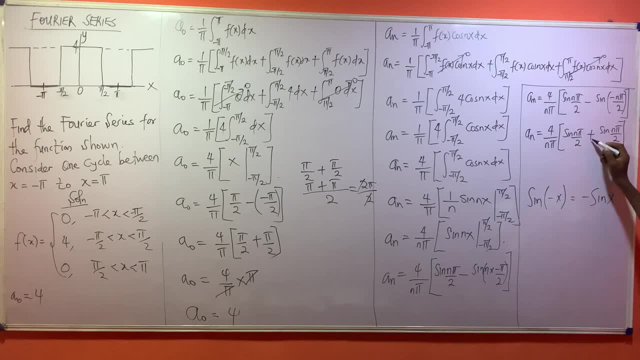 So minus minus will then give us what A plus. So that's why this guy Is a plus there, That is why it is a plus. So let us proceed. This will become a sub n equal 4 over n pi. Then you have sine n pi here. You have sine n pi here. This will be giving you 2 sine n pi over. 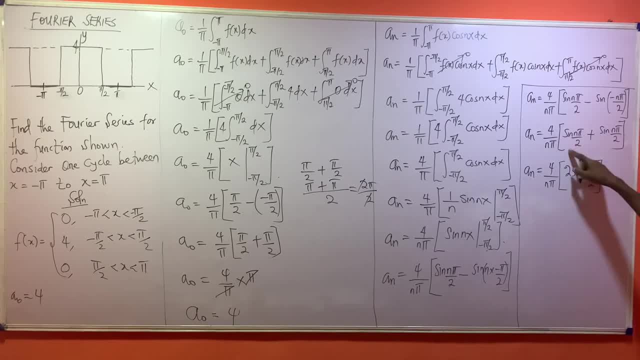 2. Because they are both the same. They're actually the same thing and they're adding themselves. So there's an invisible one here, Another invisible one here. That will give you 2 sine n pi over 2. And this a sub n equal 4 over n pi. Do you agree that this 4 and 2 can multiply? 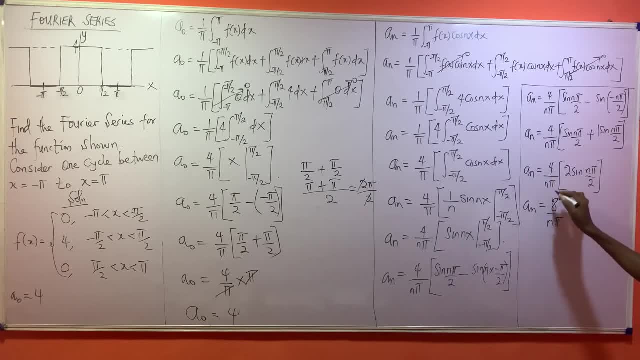 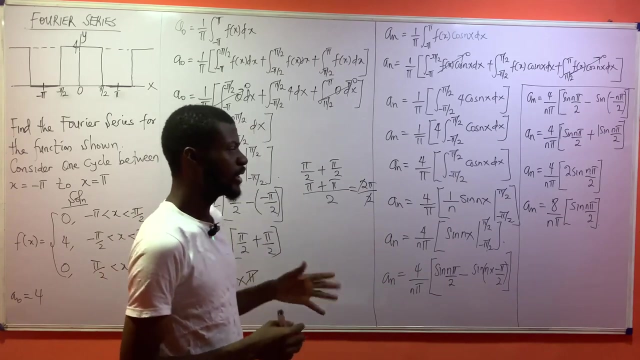 Obviously, they can multiply, and this will then give me 8. Then I'll be left with what Sine n pi over 2.. Okay, Now, that is all for a sub n, Though we do not end there, We will try to do. 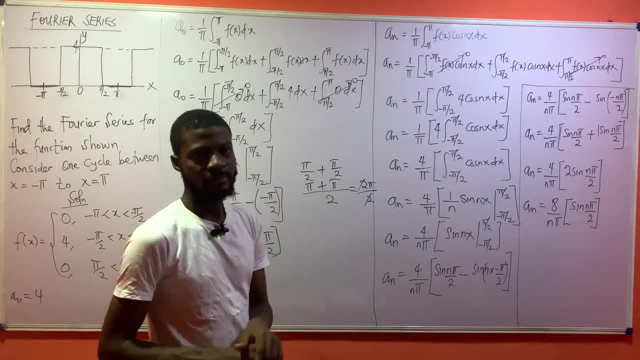 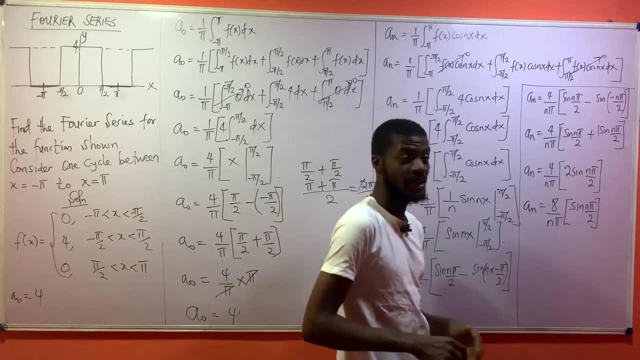 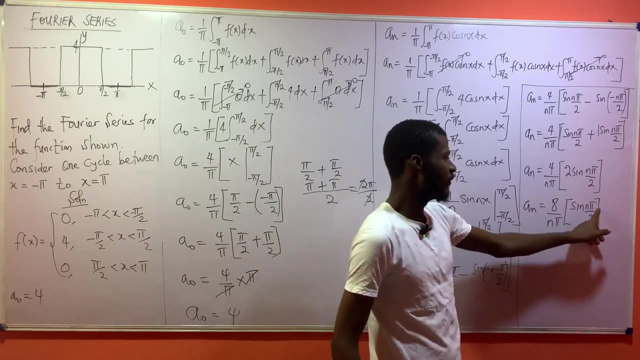 something here. We'll try to do something. That's our a sub n. We can't really calculate much, But we want to find out the pattern this is going to follow If we pick values for n. The pattern this is going to follow. Now see Pi over 2.. Pi over 2 is 90 degrees. I hope you get that, Because 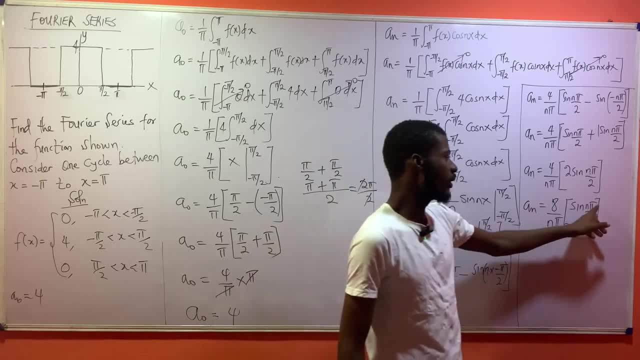 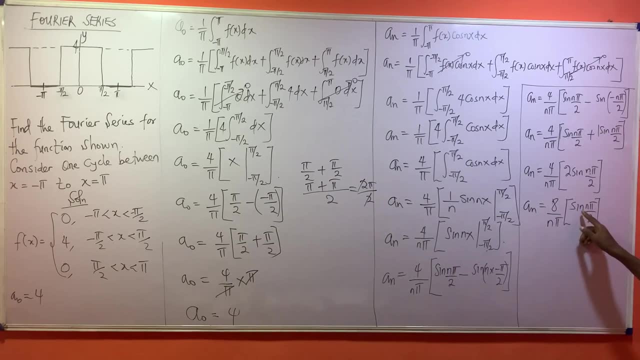 pi is 180 degrees. So 180 degrees over 2 will be giving us 90 degrees. So imagine if we pick n value as 1.. Sine 90 is what 1.. So these values are going to change. Let me just come to this part of the board to write that 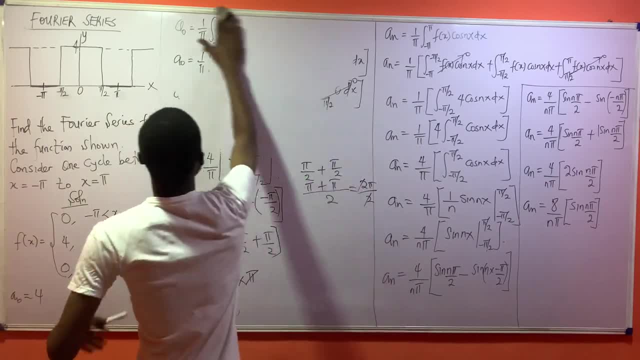 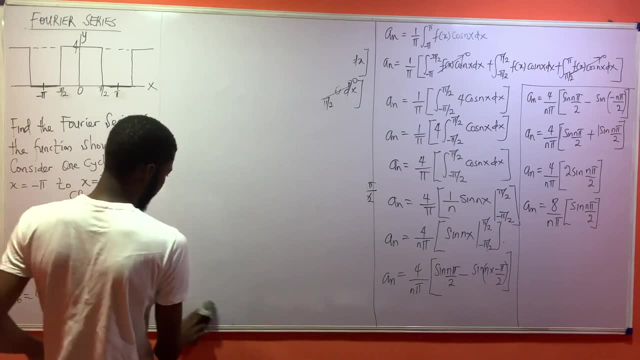 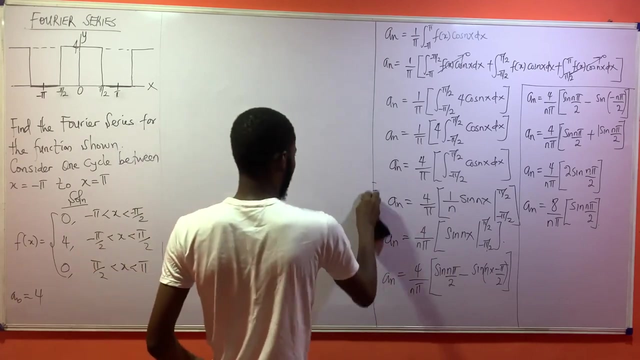 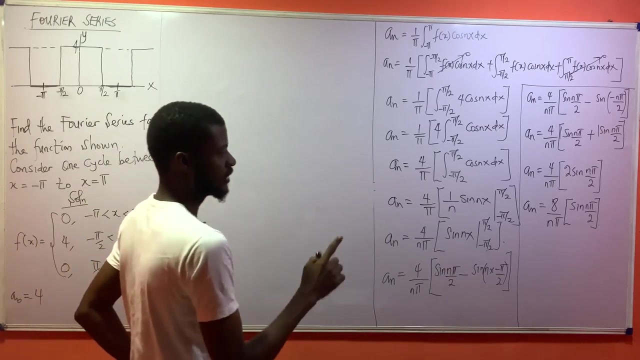 down And let us see how it follows a particular pattern, Because when it gets to that very part, it's going to follow a particular pattern. It's going to follow a particular pattern. Okay, Let me wipe this very guy off. Okay, Now look at this, Look at this, Let us find something. 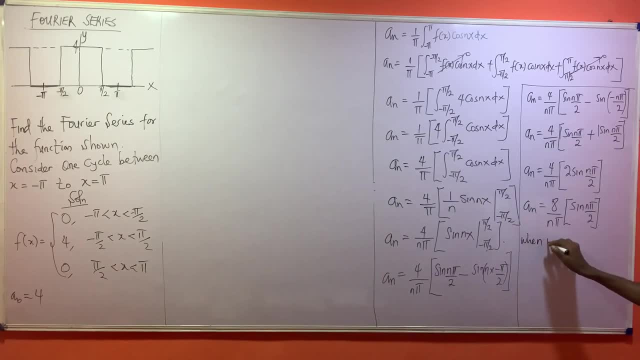 Let us say When n is equal to 1.. When n is equal to 1. Is an illustration For us to find out how the sine guy, Sine pi over two affects our result. So when n is equal to 1.. I am only concerned about this very pattern. I'm only concerned about this very 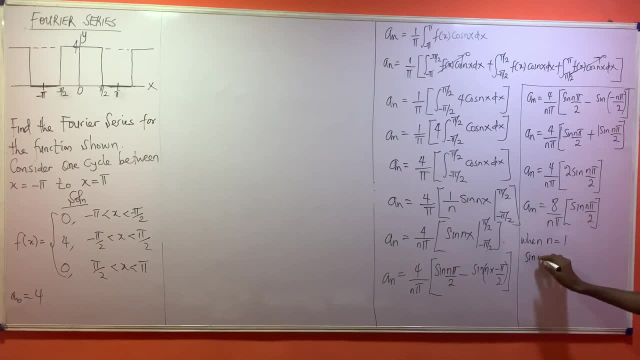 part. So that means sine n pi over 2.. Will become sine pi over 2.. Which is equal to what? 1? look at it here: if your n is equal to 1, n is equal to 1, 1 times anything is worth that same. 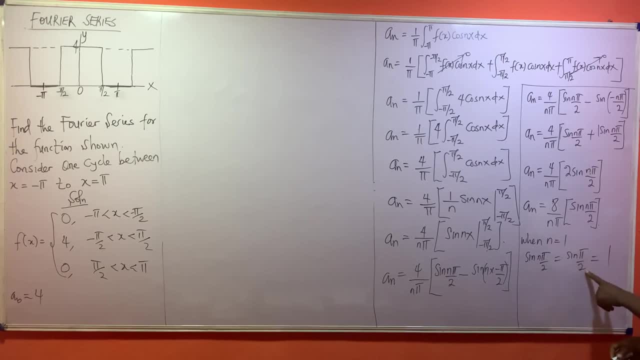 thing. so this is sine pi over 2, and what is sine pi over 2 is equal to what 1. so this is what we have. this is equal to what 1. this guy is equal to 1 because pi over 2 is 90 degrees, and 90 is what. 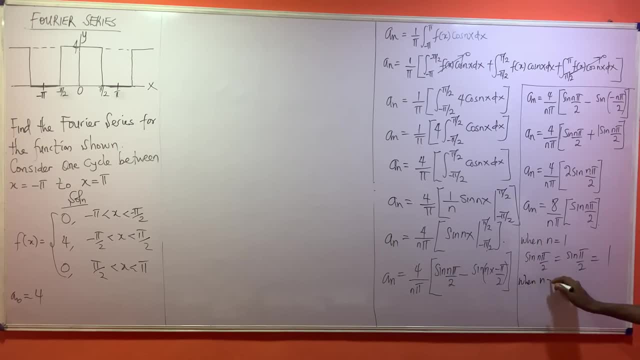 1. now what if? when n is equal to 2 and i say that this is sine n, is 2 right. so this is 2 pi over 2, so 2 can cancel 2. here we say that this is sine pi. and what is sine pi? 0. 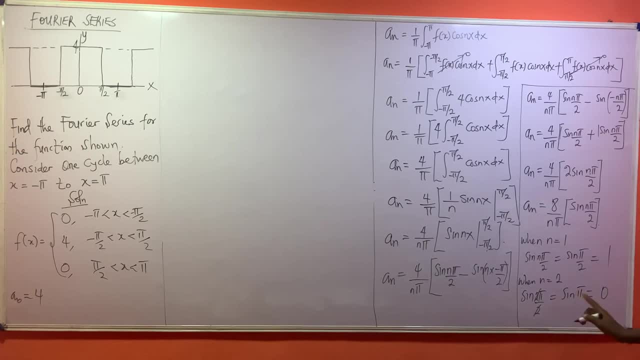 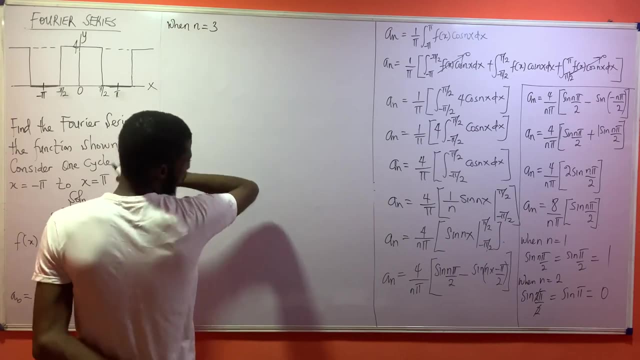 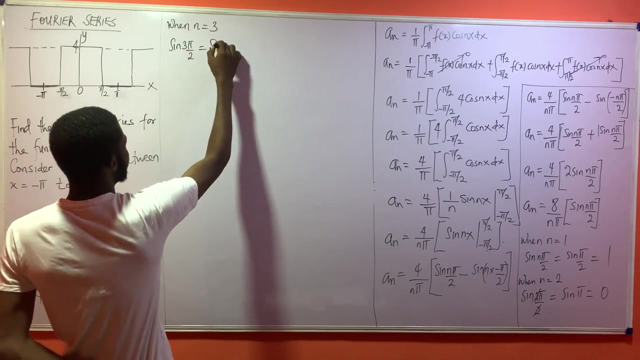 because sine 180 degrees is what 0. this is getting very, very beautiful. then also, when n is equal to 3, what would then become the value for that? i can say that i will have sine 3 pi over what 2. i can do this. so this is sine. what is pi over 2? on a normal day, pi over 2 is 90 degrees. 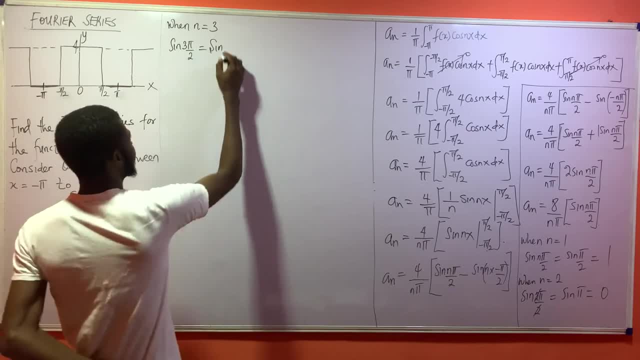 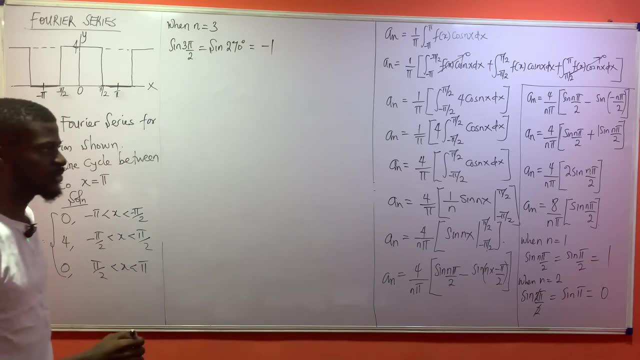 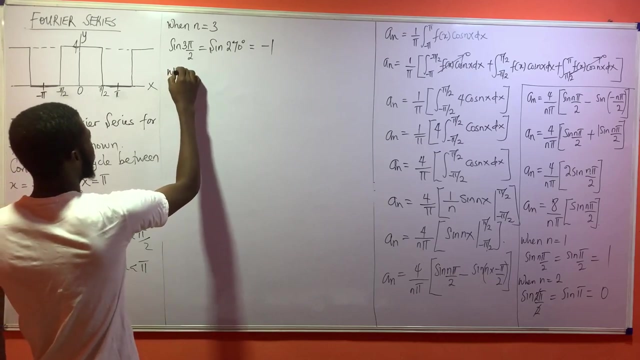 so 90 degrees times three will be giving us 270 degrees. 270 degrees, i will sign: 270 degrees minus one, minus one. okay, now, at this very point, at this very point, if you continue to, when n is equal to four, which is even your answer, this is even right. your answer is going to give you. 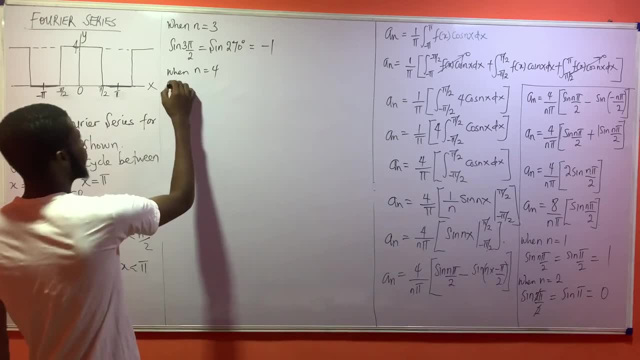 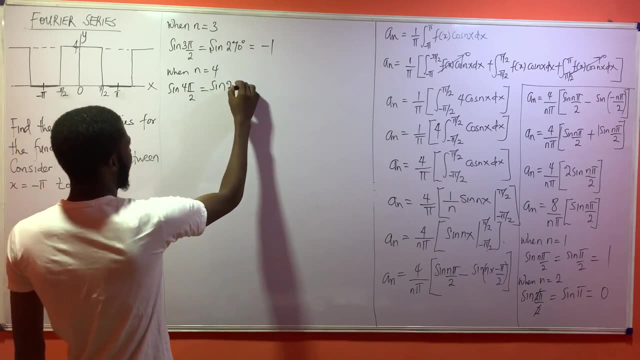 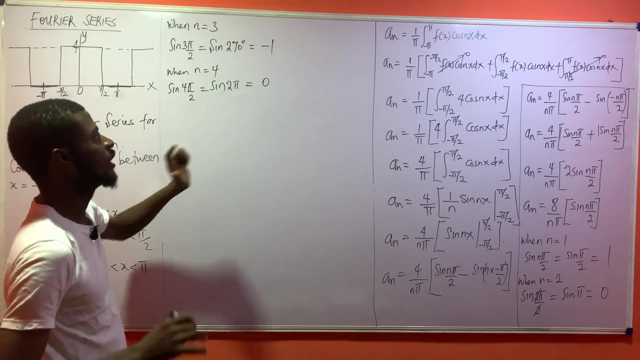 zero. so you might want to let us try that. let us see: sine four pi over two. this will become sine four over two is two, right, so this is two pi. the answer for this is still zero, because sine 360 would always give you zero. now you can conclude. if you wish, you can conclude. 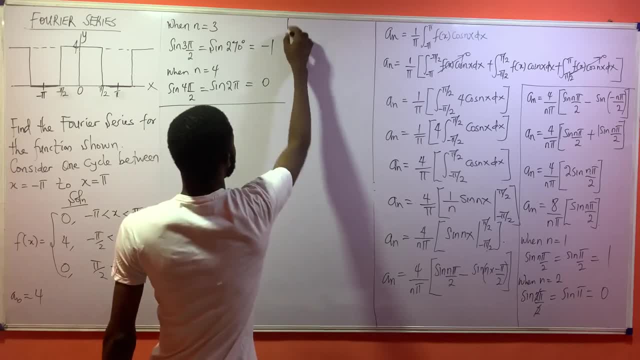 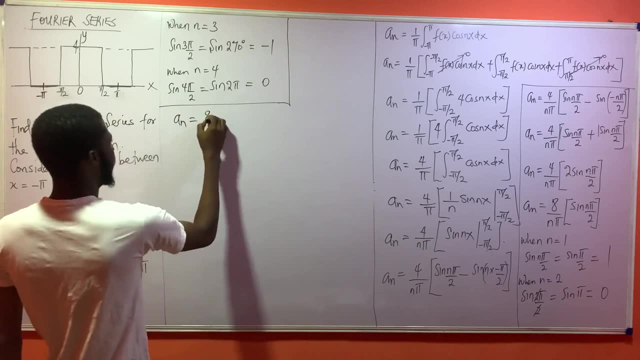 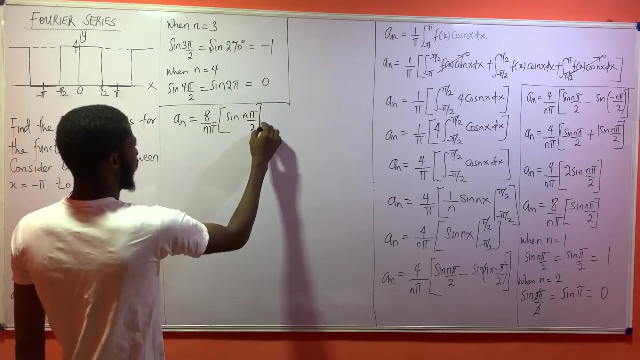 that to start with, to start with, to start with, you can say that a sub n is equal. what do we have there? a sub n is equal to zero. a sub n is equal to zero. eight over n pi bracket sine m pi over two. this is what we have right? so i would say: 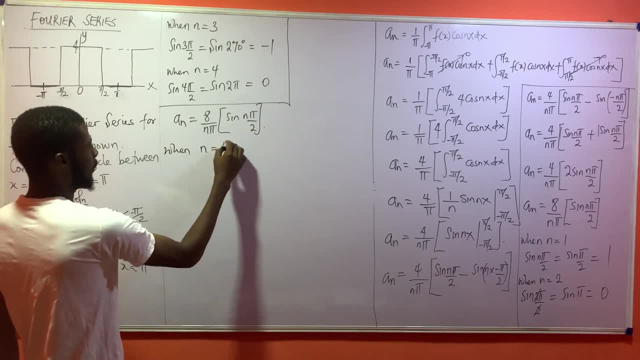 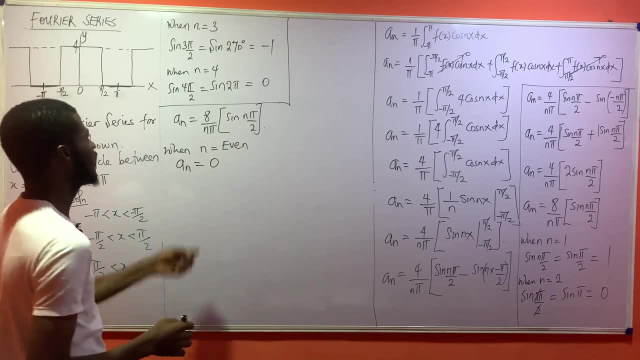 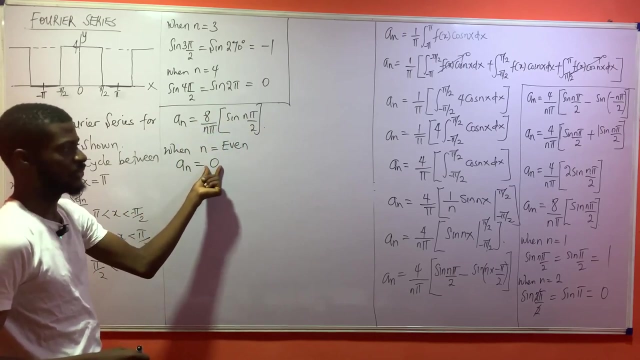 when n is even, when n is an even number, when n is an even number, i will say that a sub n is equal to what zero, because we can see that this is an even number. our answer for this very bracket is: what zero? so zero times. this will still give me zero. same thing happened here when n was. 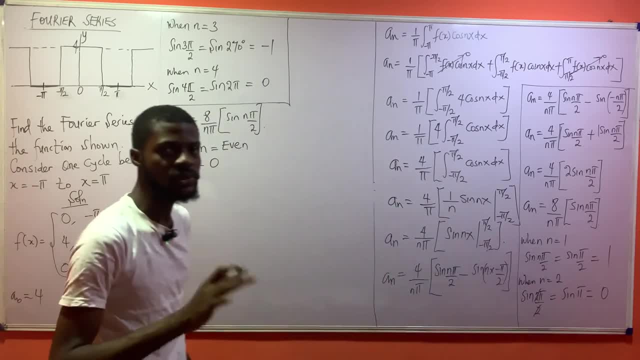 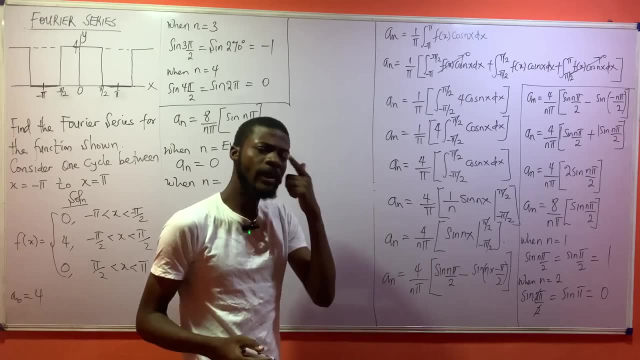 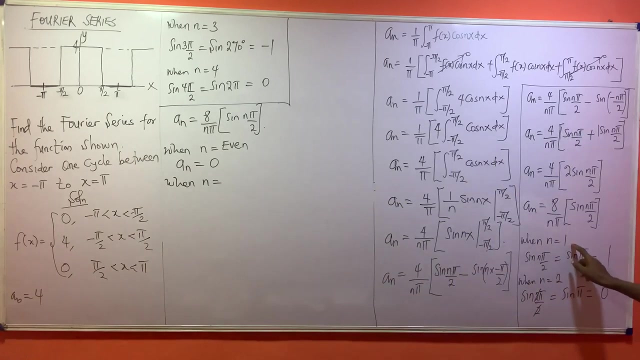 an even number. this very part gave me what zero, so it's kind of easy. the next one is when n is equal to an odd number. but the problem here is this is a problem here i cannot just say odd numbers, because we notice that when n is equal to one, here our answer for this bracket was one which is an odd. 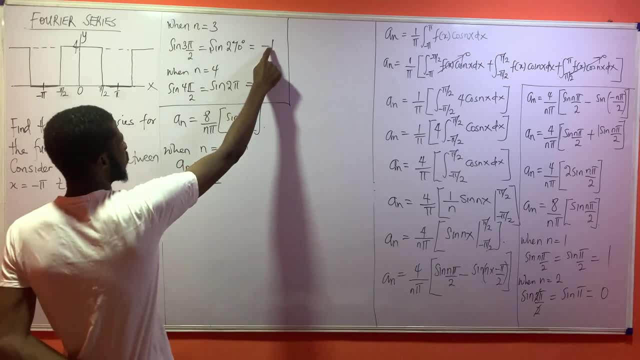 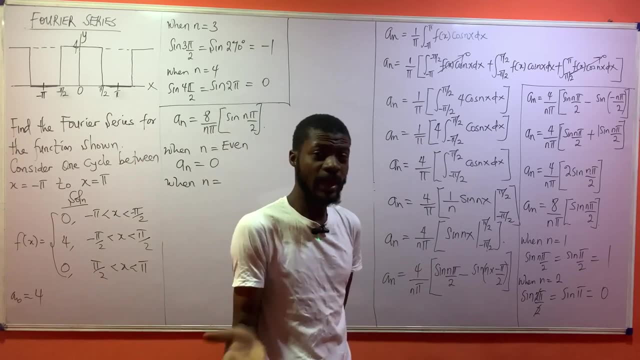 number. now, when n is equal to three? here the answer was: what minus one? so you can see that it's going to be interchanging between one and n is equal to one, so we can see that it's going to be interchanging between one and minus one. one and minus one, even though they are both odd numbers. 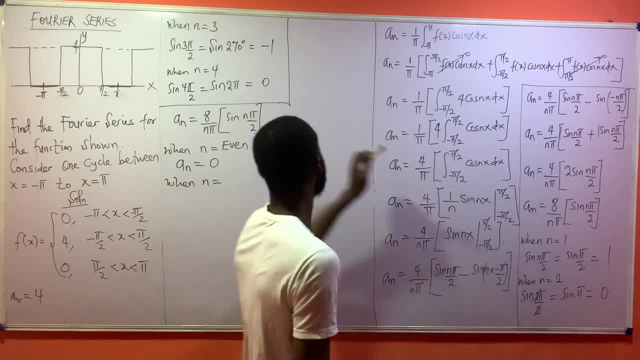 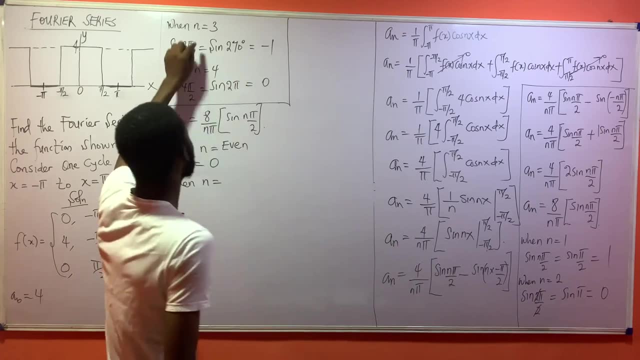 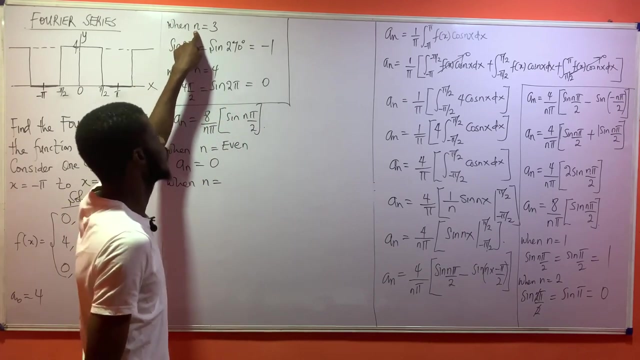 because n equal to one is an odd number, then n equal to three is also an odd number. now, how do i know this, or what do i then say? is this relationship? if n is equal to three? here, and my answer for the bracket is: give me minus one, what other odd number, or what is the closest odd? 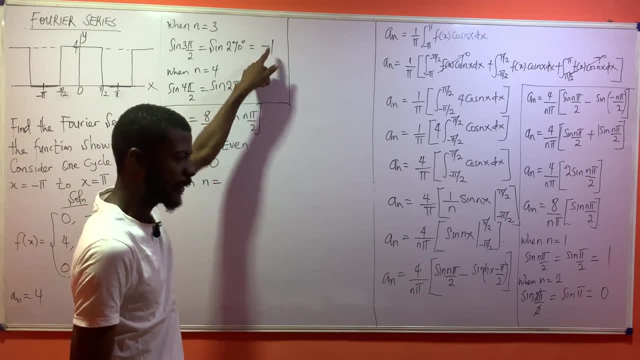 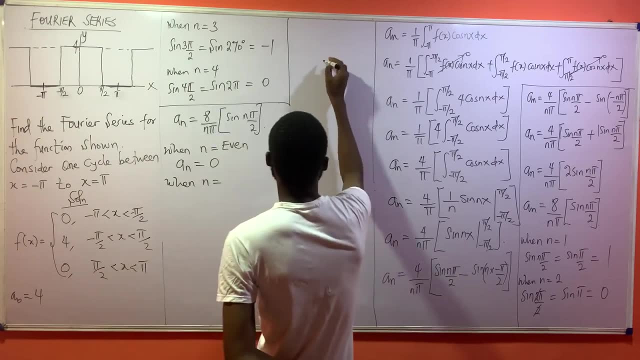 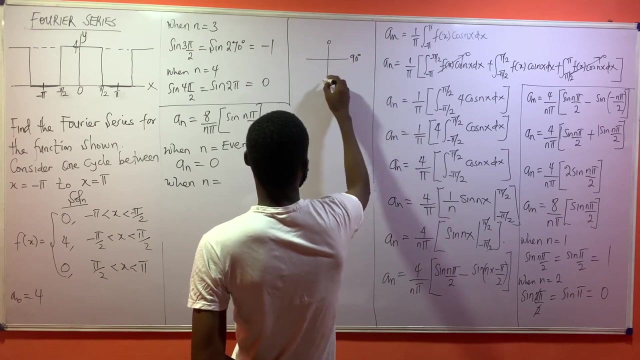 number to this very three, that will give me the same minus one. now look at it this way in. okay, let me see, i'll focus on it now. point for cardinal points. let me draw this very guy. i think i like drawing this. we have zero, we have um 90 degrees- i think i'm drawing this one 180, we have them 270 and then 360 degrees, something. 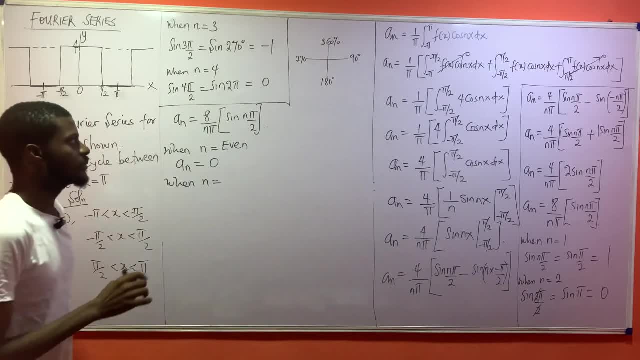 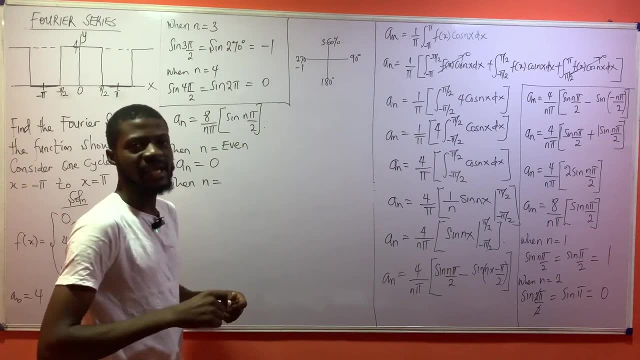 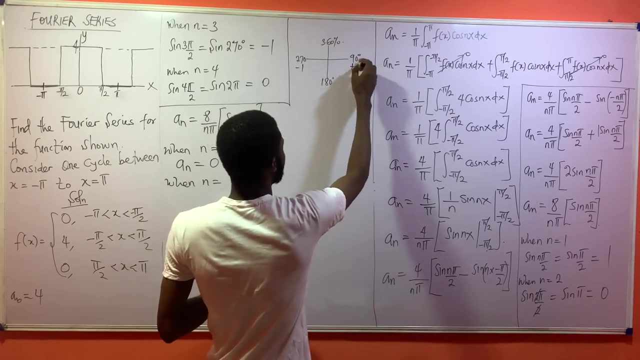 like this: okay, now this very part holds minus one. i think did i even draw this correctly. this very part is minus one. now the next minus one will come up when it comes to this very location again, because this is minus one and this plus one, this the the next value i'm going to have that will. 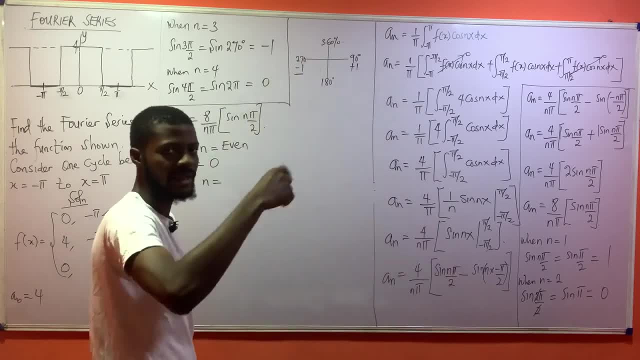 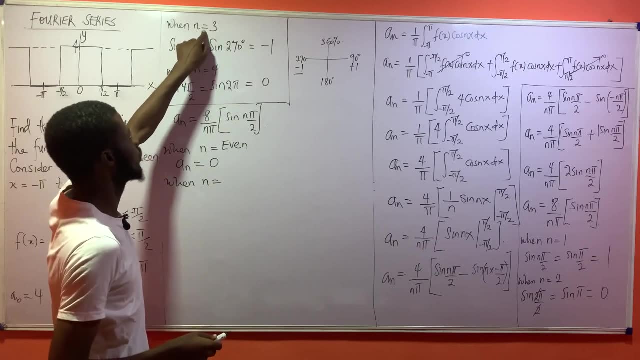 give me minus one is going to come around again. so i'm going to be having like a 360 degree tone and that's four, that's four. so if n is equal to three, n is equal to three. for you to give me minus one, it means that the next minus one i'll be getting is when n is equal to what. 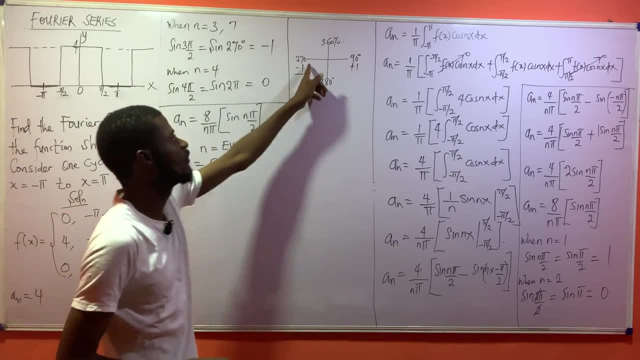 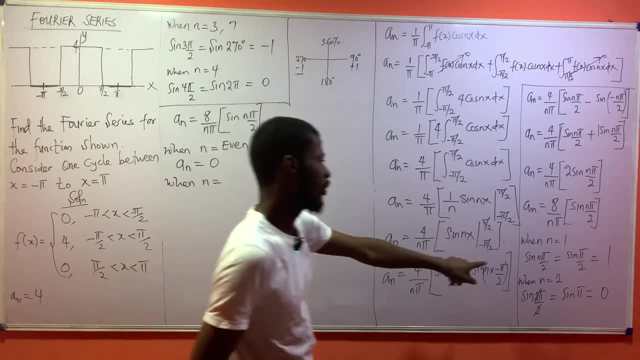 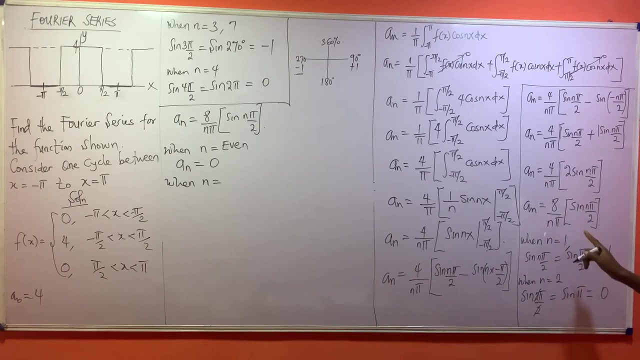 seven. that's the meaning, because i will have to move four times from here to here, here to here, here to here. then move here again for me to see minus one same thing is going to happen here if n is equal to one here. the next time i'm going to get one is when this thing moves for um distances. 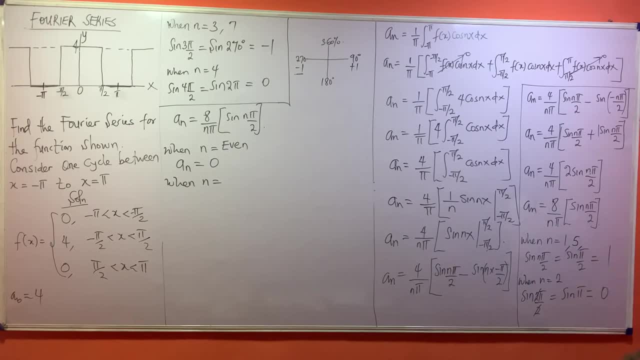 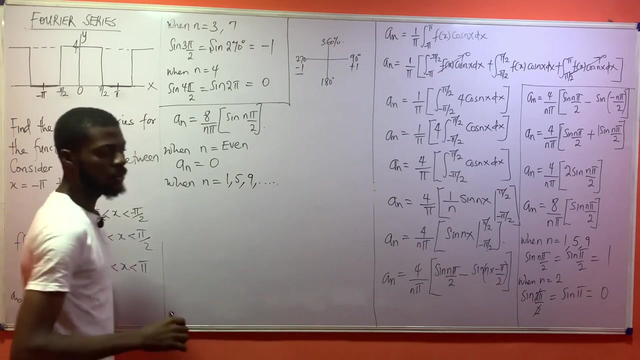 so this is going to become what one plus four is what five. the next guy: five plus four is what nine. so this is just it. i don't want to go that much. so when n is equal to, let me go with that one: five, nine, then continuously. what do you think of my answer when n is equal to one? 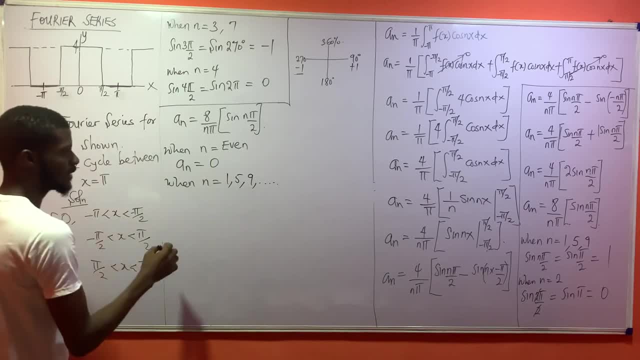 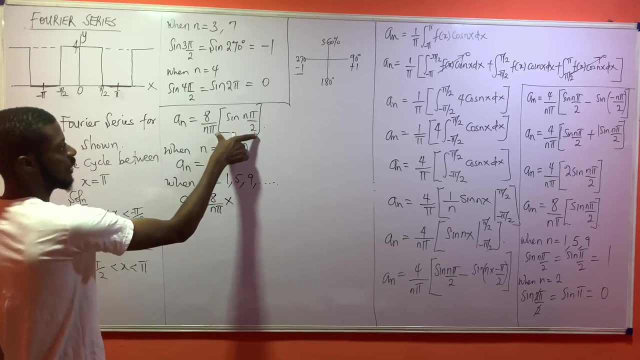 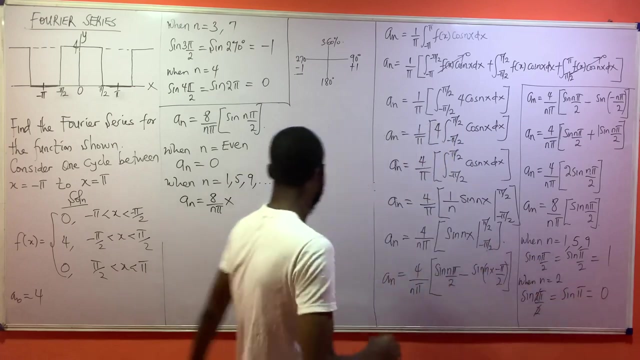 five, nine, what is it could then become my answer now: a sub n is equal to eight over n pi times. what is the value of the bracket at this very, at these very types of numbers? one, five, nine? the answer is what one? so i'm going to say times one. so this: a sub n equal anything, times one is that. 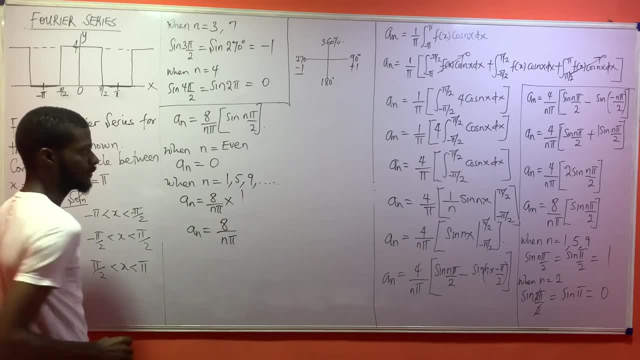 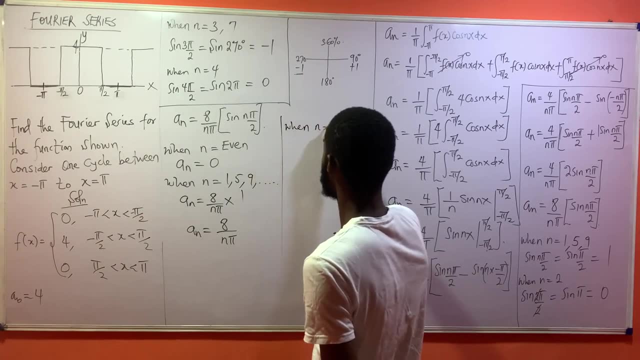 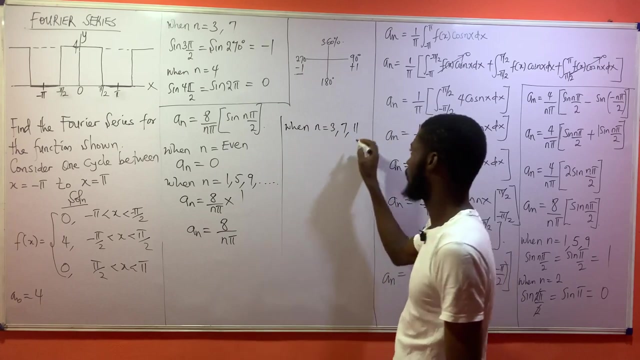 same one. so i'm going to say times one. so this: a sub n equal anything, times one is that same one, same thing. so this is eight over n pi, very sweet. then the next guy. when n is equal three, seven, what are you talking about? the next guy here: eleven, because we're always adding four. okay, 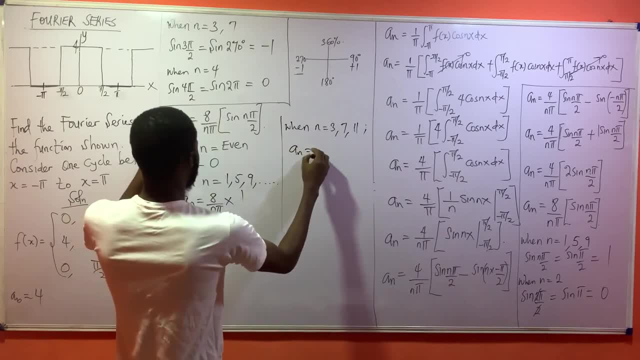 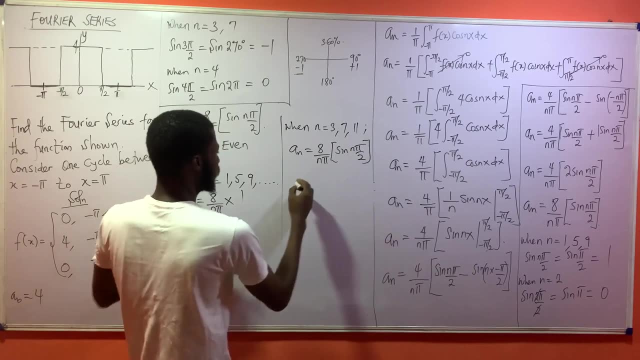 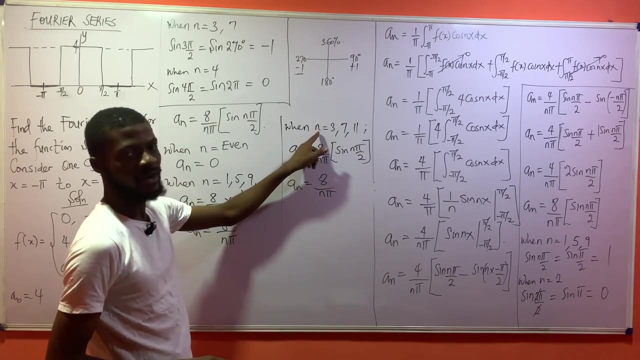 it's. it's very simple. so this is a sub n equal eight over n pi. then bracket sine n pi over two, so this a sub n equal eight over n pi. now, what is the value of this very bracket when the numbers are of the form three, seven, eleven, and what have you when it's of this very form, the value. 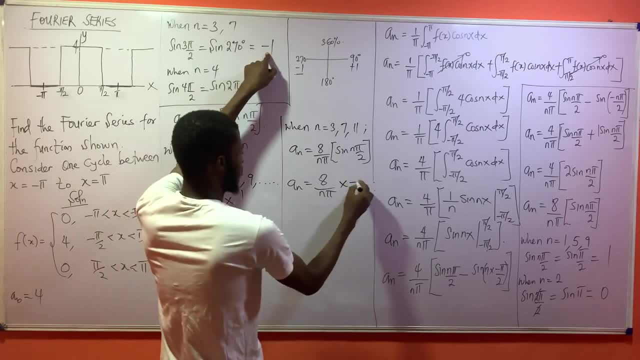 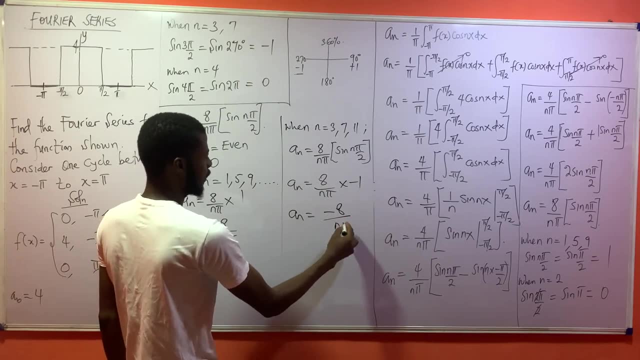 for the bracket is what minus one. so this is times minus one. so that means a sub n is going to become eight times minus one is minus eight over n pi. i believe this is just the stressful part of everything. this is just stress. so these two answers are going to be the answer to the question of how. 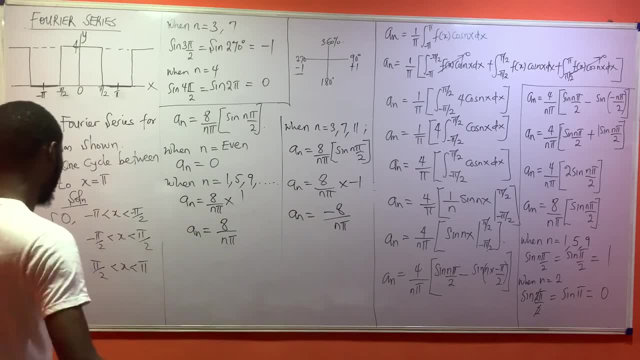 are actually going to be what written down so i can come. okay, i think i love writing my answer at this very part, so i can see that a sub n is equal eight over n pi for n equal one five, nine, something like this. then a sub n is equal minus eight over n pi at n equal three seven. 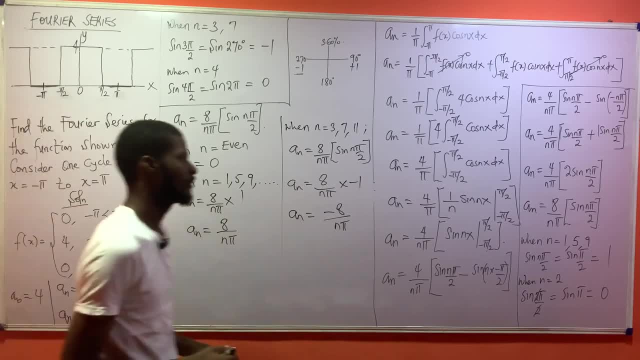 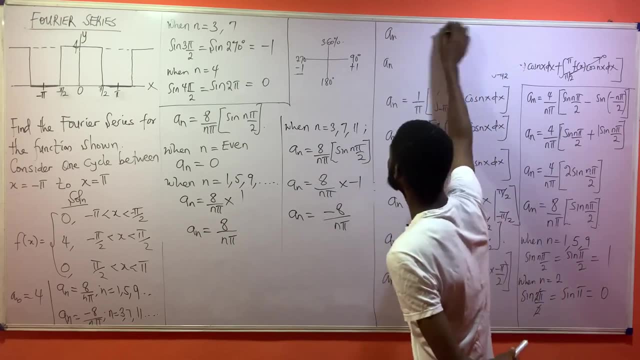 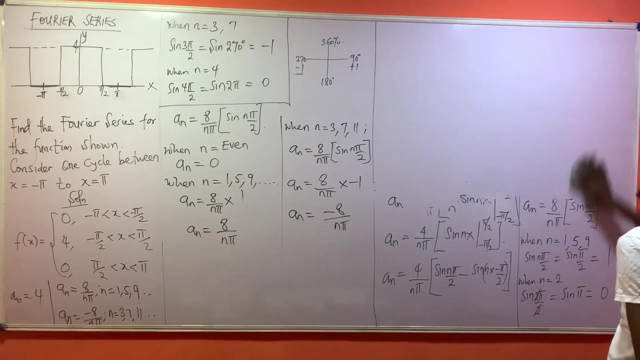 eleven. just like that, i can do that, very guy, it's possible. so let us go to the next one: b sub n. b sub n. even though we do not really need to find this sub n, but let us just find it. even though we don't need to find it, but let us just find it, there's. 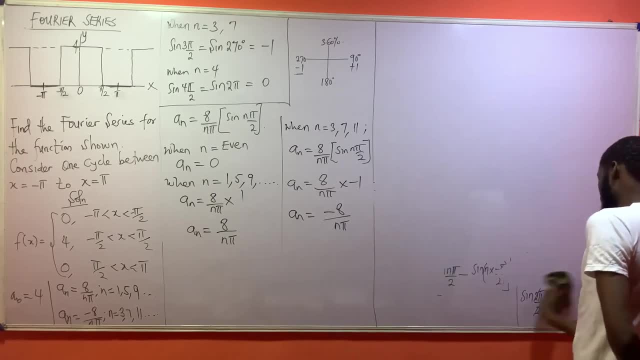 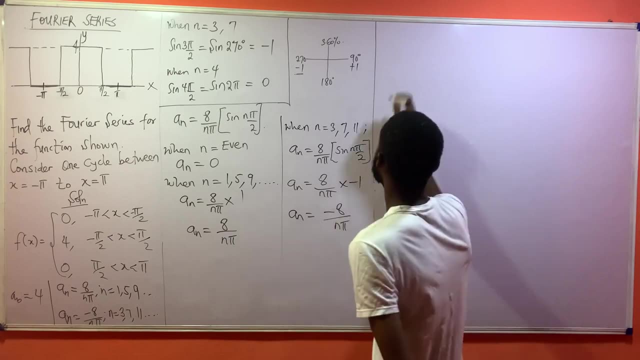 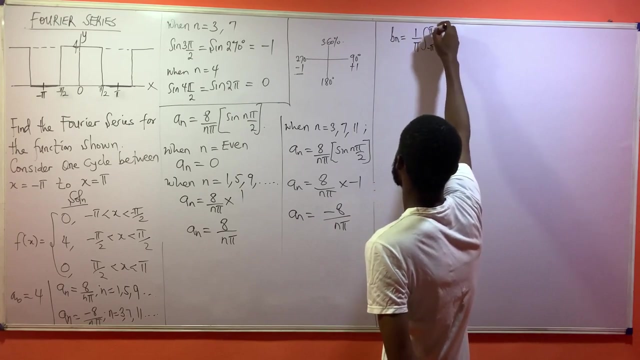 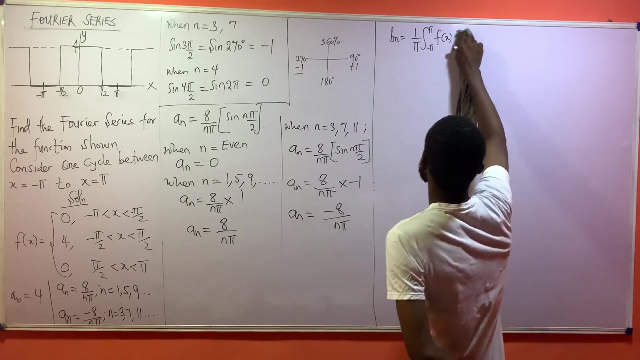 a reason why, then i would explain why you never needed to find it. okay. now look at this very guy: b sub n. b sub n is equal one over pi, integral from negative pi to pi of f of s cos. sorry, not, because it was that this is going to be sine. so this is sine nx dx. so that's what we have. 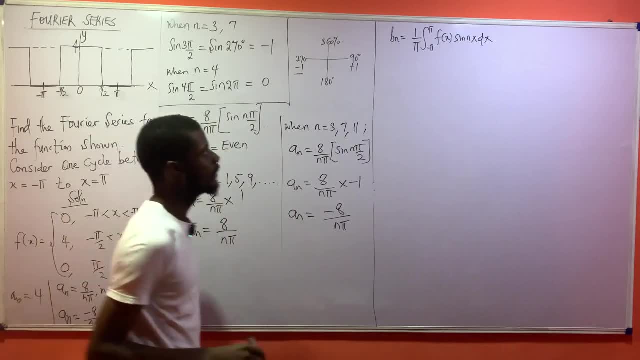 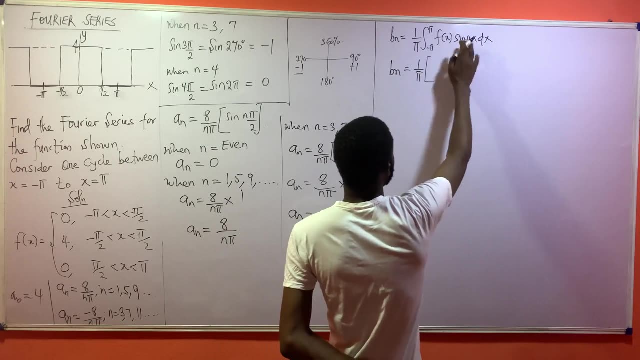 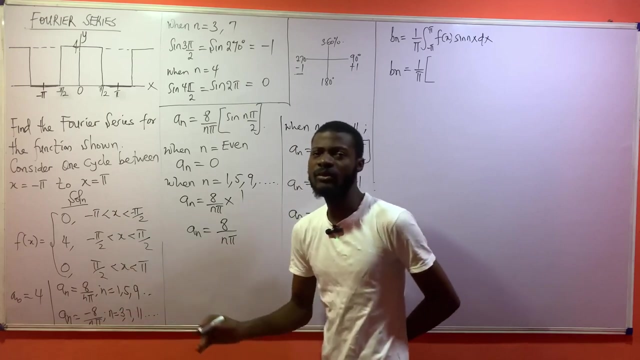 this is what we have. for what? for b sub n. now we see that this is b sub n, equal one over pi. now you would agree with me that, this very guy, i'm going to still split it like this. i'm going to split it like this: from minus pi to this, this to this and this to this, instead of me wasting my 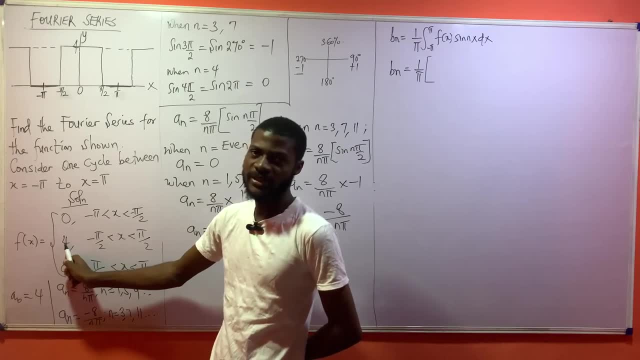 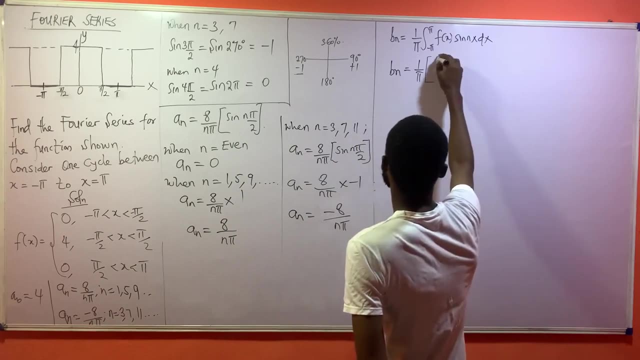 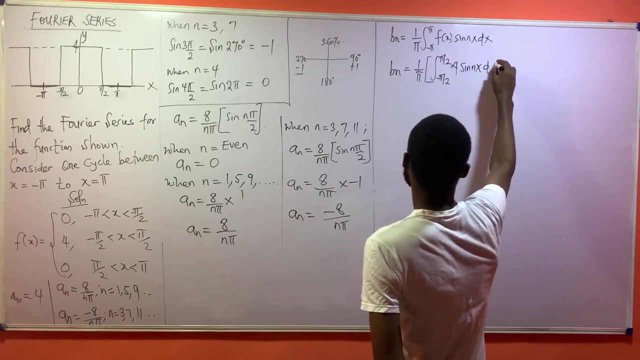 time, i know that it is only this very four that is significant, because this zero and this zero are going to cancel out. in the previous example you've seen that, so only for me to stress myself, i can say that this is the integral of negative pi over two to pi over two of four, sine nx, dx. 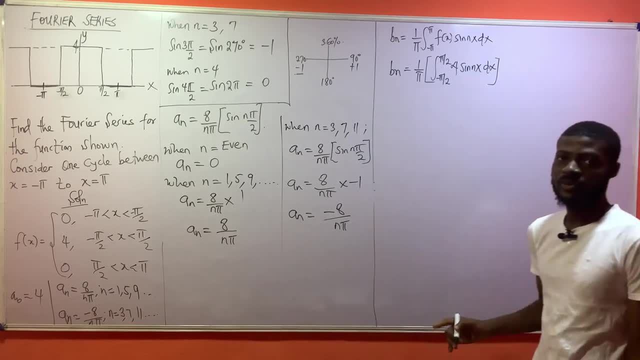 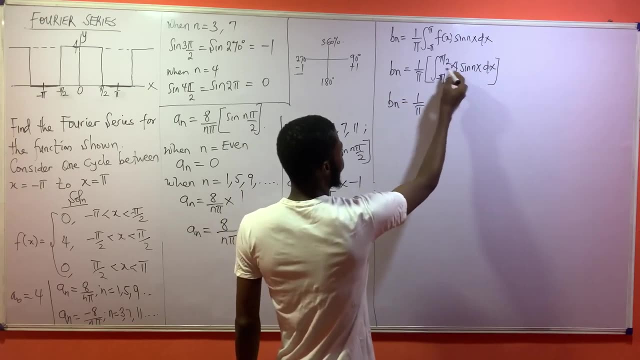 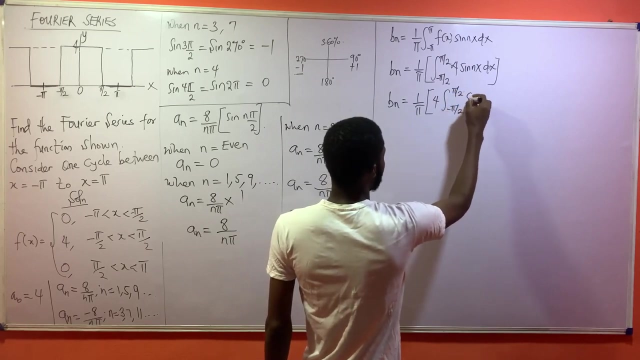 yeah, i can do that. it's possible for me to do it. so this is all correct. now this is b sub n equal one over pi. then we have this very four can come outside, right. so this will then give me four with the integral of minus pi over two. so pi over two of sine nx dx. i can actually do this. 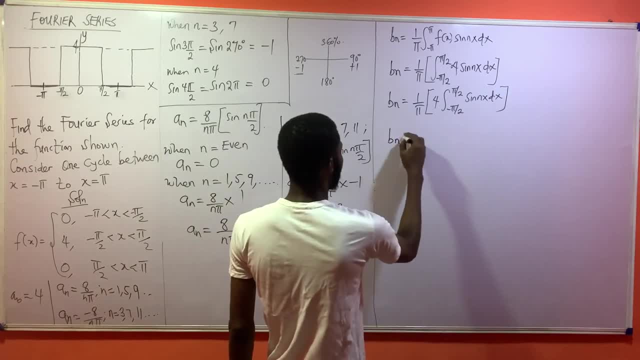 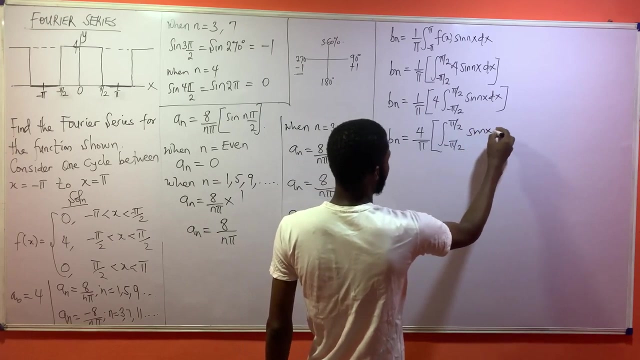 it's possible for me to do that. okay, now, this b sub n, equal one times four, will give me four. so this guy is going to be giving me four over pi, then the integral from negative pi over two to pi over two of sine, nx, dx. now let us now evaluate the sine guy. let us now evaluate it. 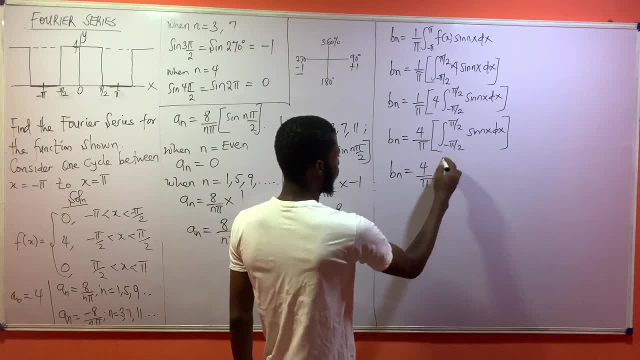 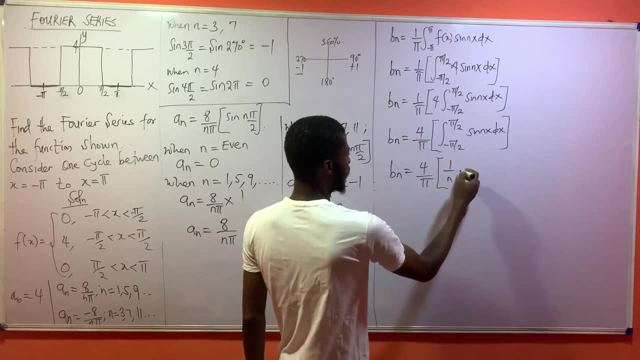 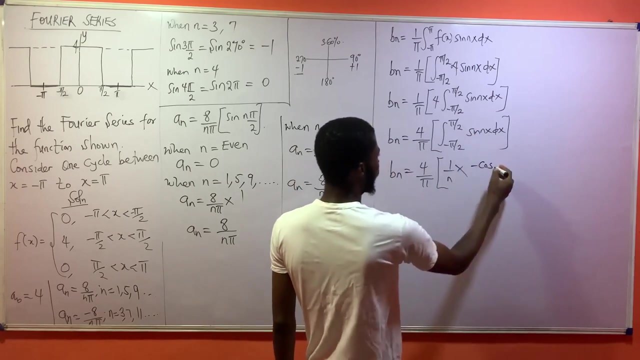 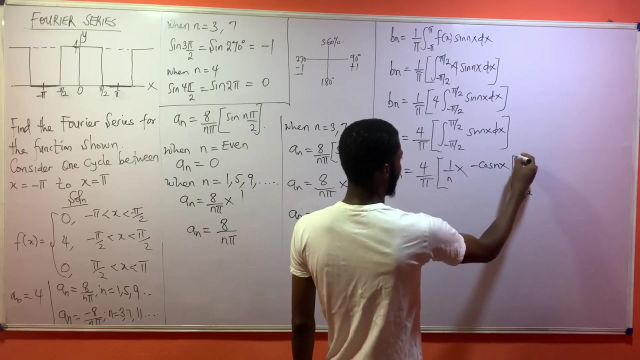 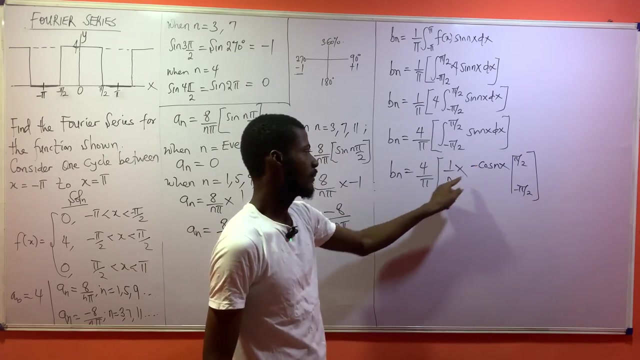 now b sub n is going to become four over pi. now differentiate this very angle: nx, what would you get n, so you're going to say one over n. then times integrate sine, what would you get? one over pi also, but this is the deutsch idea. so, okay, think that it's minus col. 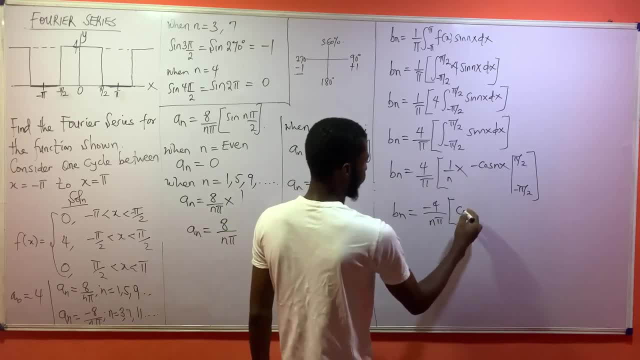 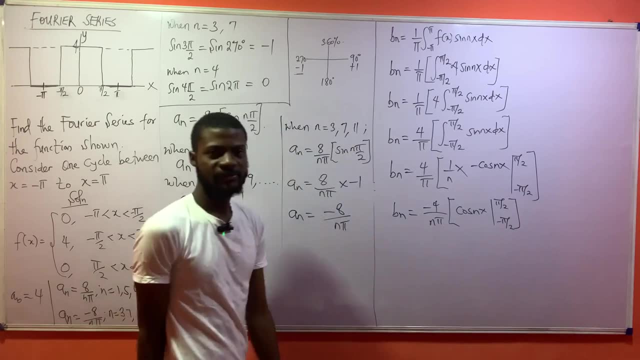 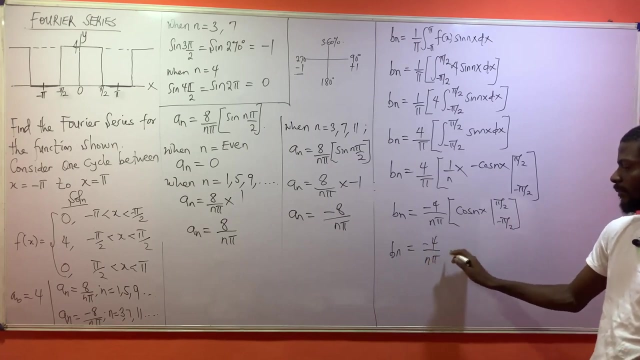 b. so then what we get: force cos nx from minus pi over 2 to pi over 2. so this is what we have now see. this is b sub n equal minus 4 over n pi. now i'm going to make two brackets. right in the first bracket, s is going to: 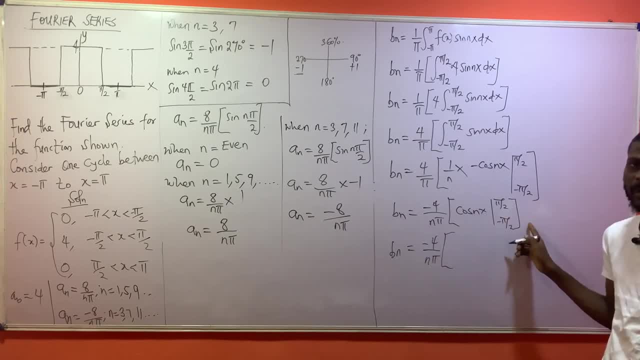 become pi over 2. second bracket s is going to become minus pi over 2, so this is cos n. s is what pi over 2, then minus. this is second bracket now. cos x is now minus pi over 2, so this is minus n pi over 2, without further ado. let us not waste too much time there if we should put x as. 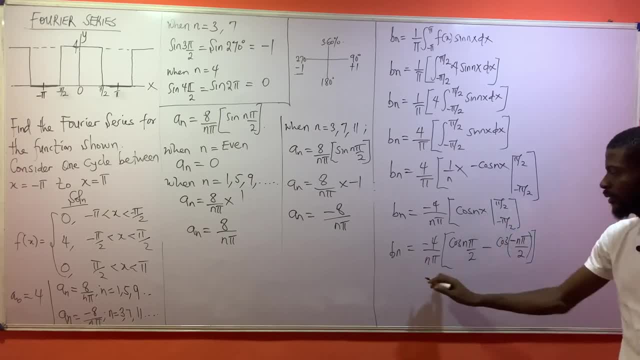 minus. so n times minus pi is minus n pi over 2. now this is b sub n equal minus 4 over n pi. open bracket. cos n pi over 2, minus cos n pi over 2, the minus can just go away. if you remember in what's it called in cosine cos. 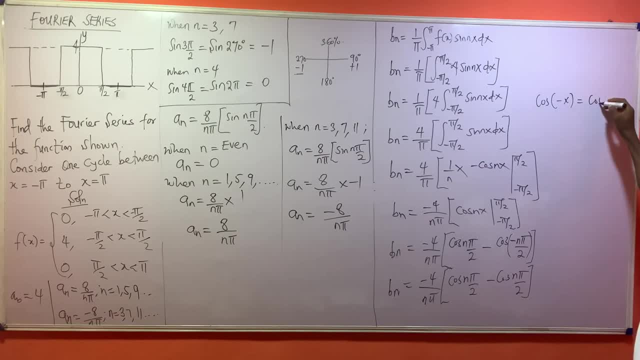 cos of minus s is same thing as cos of x. so this is for what? for cosine cos of minus s? we give you cos of x. so cos of minus n pi over 2 is same thing as cos of n pi over 2, and right now, cos n pi over. 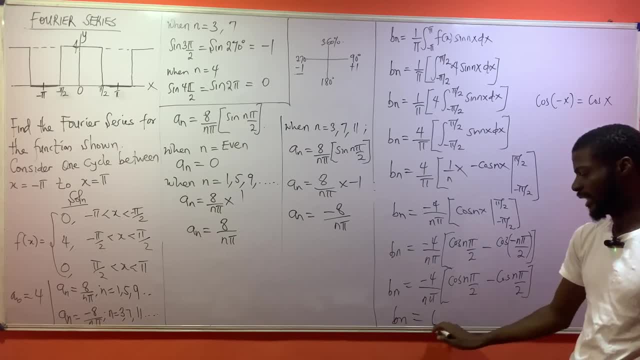 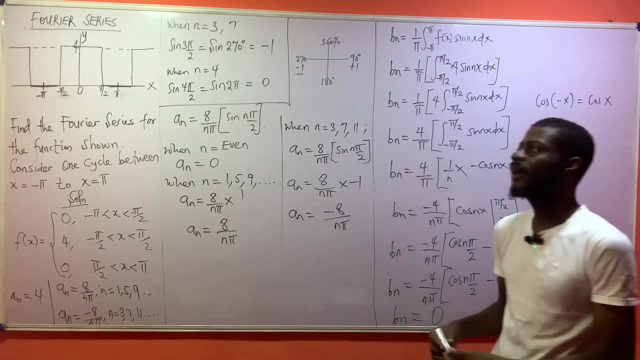 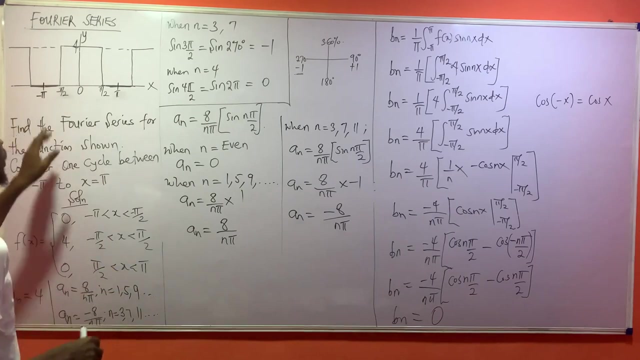 2 is the same, you are subtracting it, so this will then give you bn as what zero, because this minus will give you zero, and zero times will give you what zero, though you never. you were not supposed to do this ideally, because this very function is an even function, but we'll talk about that later. 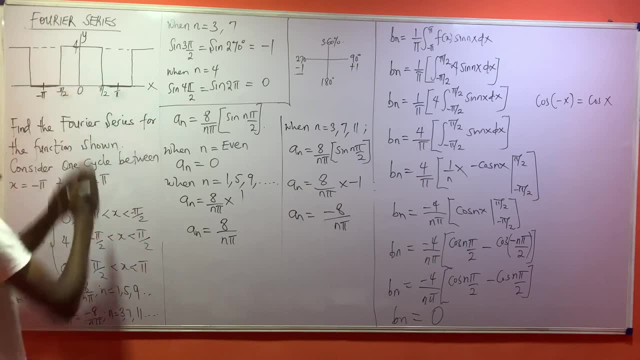 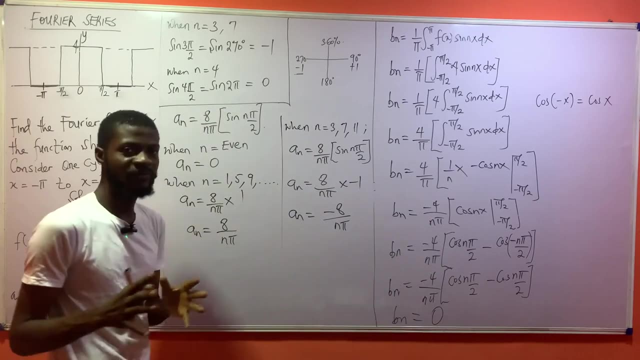 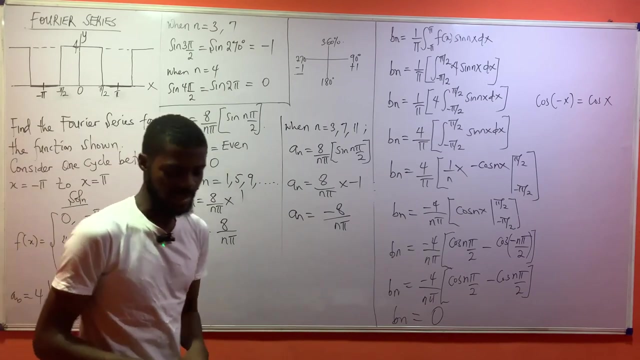 yes, it's even this part and this part can just yes, so it's an even function. but not only for us to start stressing ourselves over that. we'll do that in the um, future, in the future. so, right about now, let us get our fourier series, because we're at our final answer. 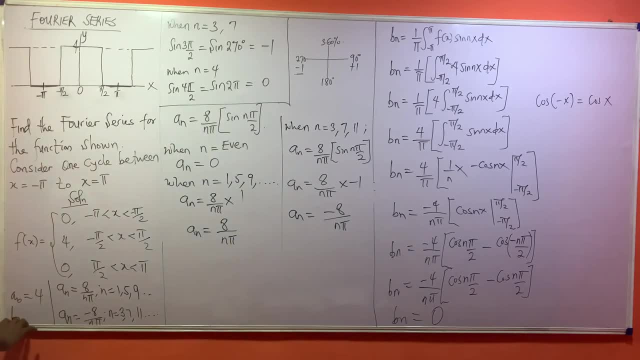 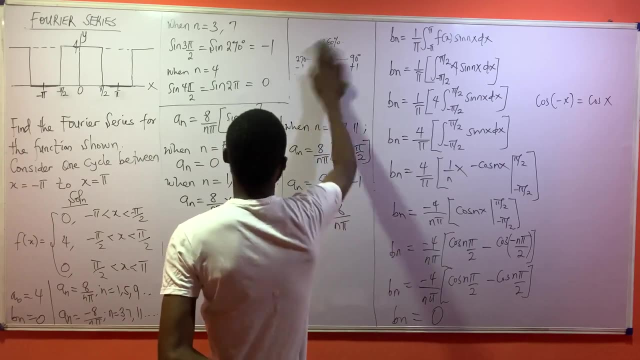 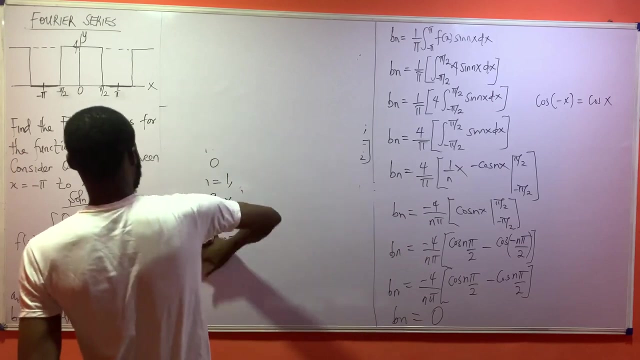 so, after getting our um b- sub n is equal to zero- and after getting all our answers, let us now get our fourier series. now i can wipe this part off, i can wipe this very part off, i can take this part out and i'll say, i'm going to say that 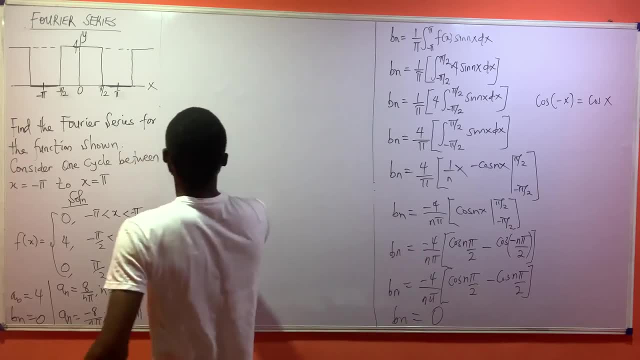 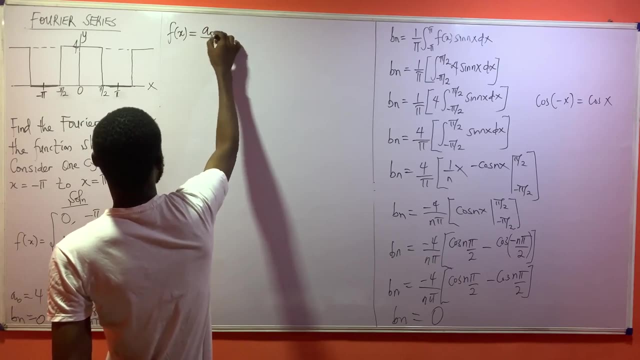 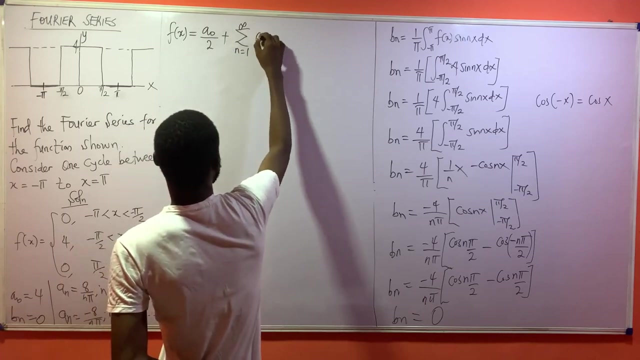 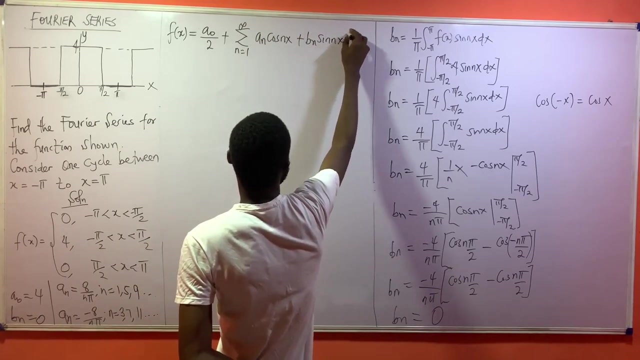 what is the formula for fourier series? f of s is approximately equal to a naught divided by two, plus summation from n equal to one to infinity of a sub n cos nx plus b sub n sine nx. so i can do this and see that this guy is what correct. now 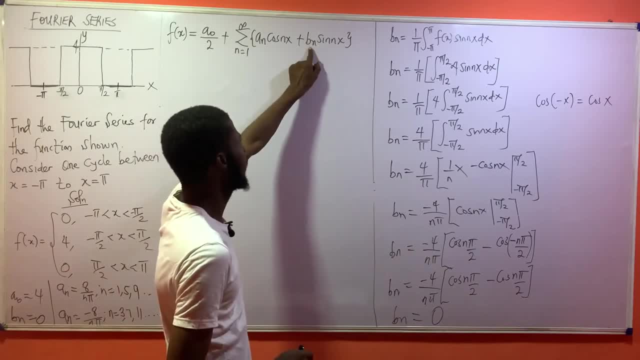 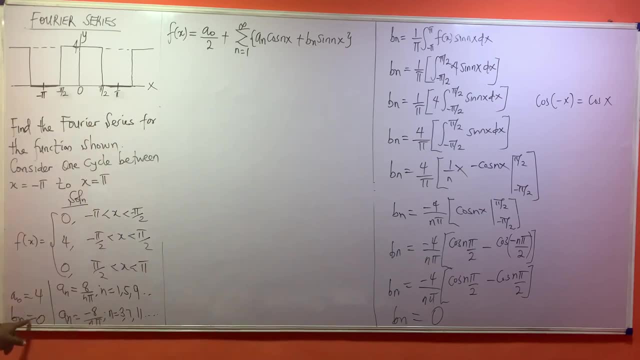 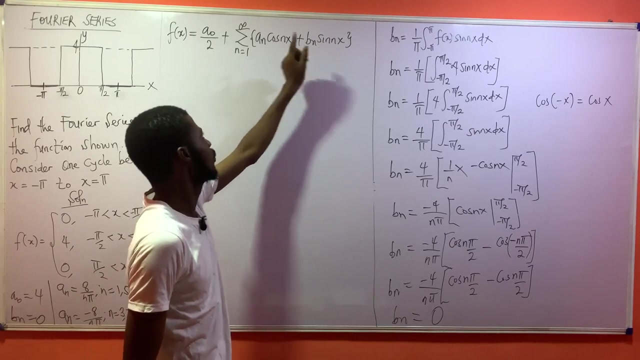 we follow this carefully, you would agree with me that this guy will. everything here will become zero, meaning there are no sine things, there are no sentences, because b sub n is equal towards zero. so this part will just go away, because there are no sign themes. we don't have sine times yet, so we have only cosine times, and cosine is an even function. 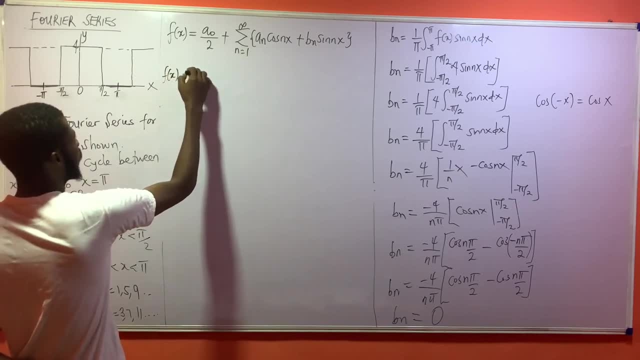 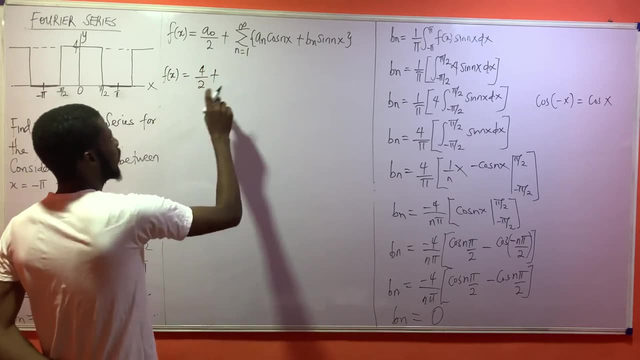 okay, now f of s will be equal to what is a naught. a naught is four, right? so this will be giving me 4, plus the summation of this very guy. Now see what I'm going to do here. Remember I said something. 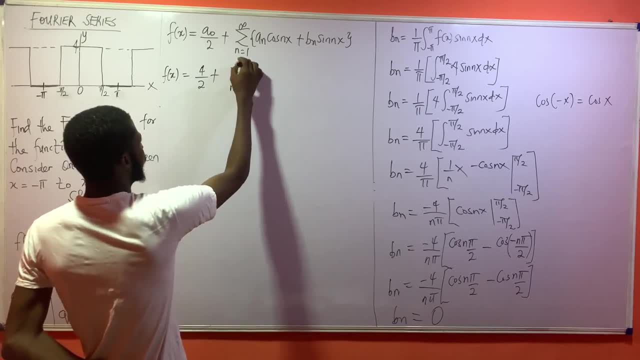 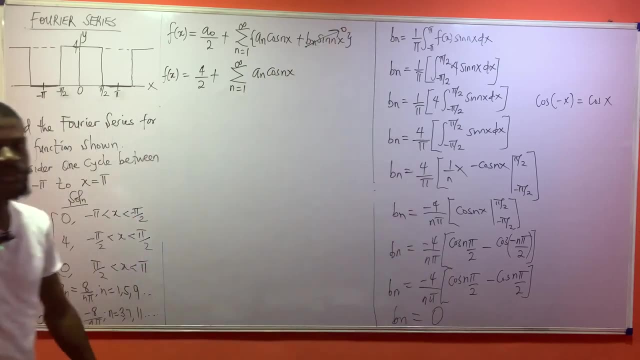 Let me just write this: The sum from n equal to 1 to infinity, of a, n, cos, nx. That's because this very part will just give me 0. It's just going to give me what 0. That's just 0.. 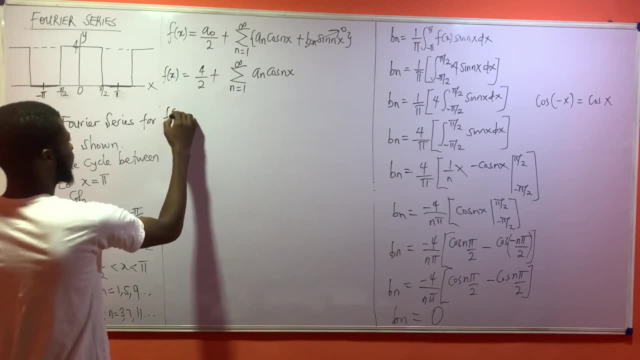 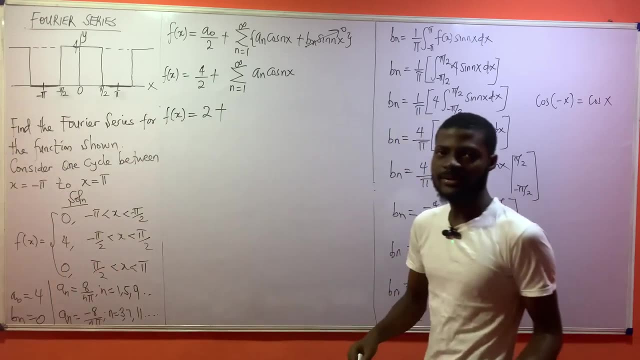 Just 0.. Okay, So this is f of s equal. 4 over 2 is 2, right Then plus. this is where we then get started. This is where we then get what Started. Now a sub n. 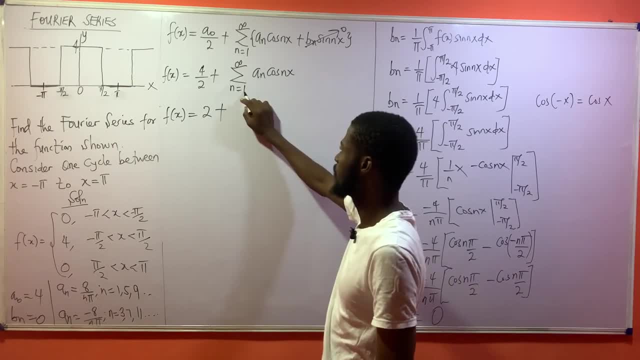 Let us start with n equal to 1.. Let us start with n equal to what? 1.. Now, when n is equal to 1, what do we have for a n? We'll be having what? 8 over n pi right. 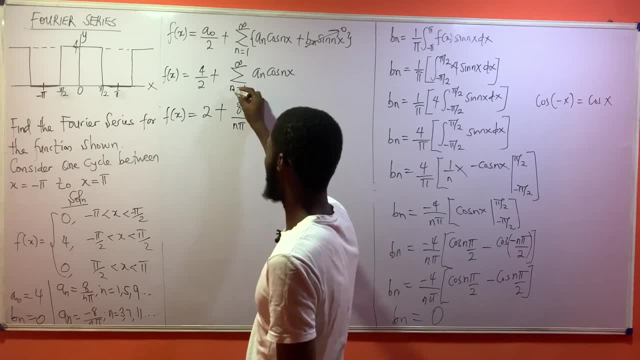 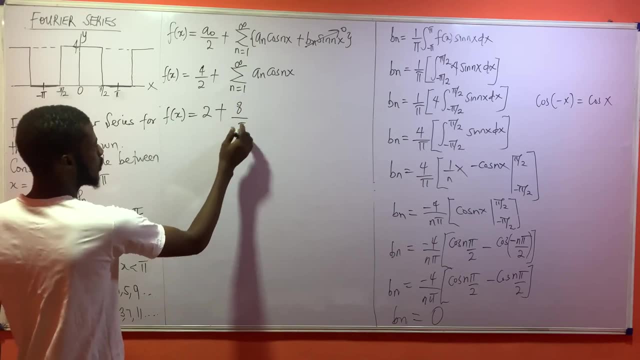 So if we have 8 over n pi. remember we said n should be equal to 1.. n should be equal to 1, right? So this is going to become. this guy is going to become what 1 pi. 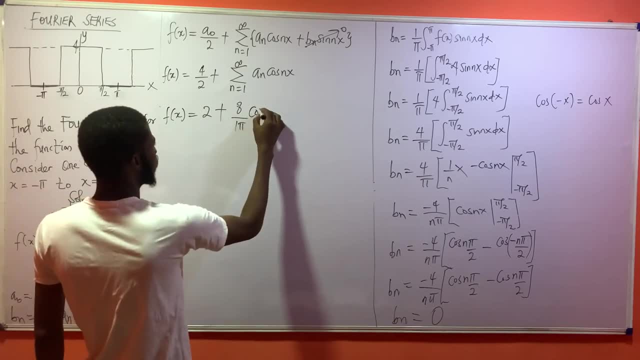 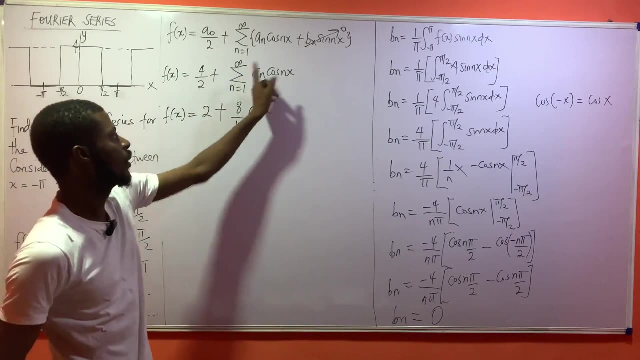 Or you can just say pi, And this is cos nx, and my n is worth 1.. So this is just cos x. So this is the value of everything here: when n is worth 1.. We proceed to the next one. 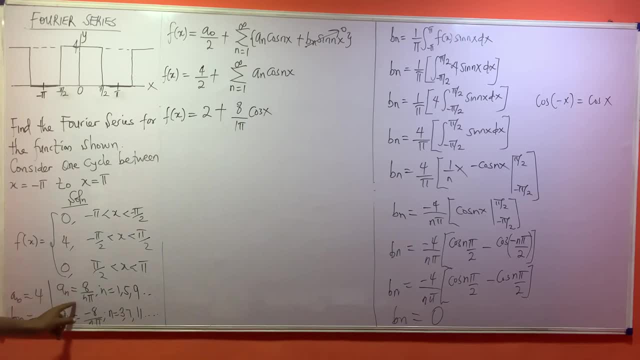 When n is equal to 2.. But the thing is, when n is equal to 2, what will happen? We have 0, right, a sub n will be giving us 0. So for even numbers it doesn't exist. 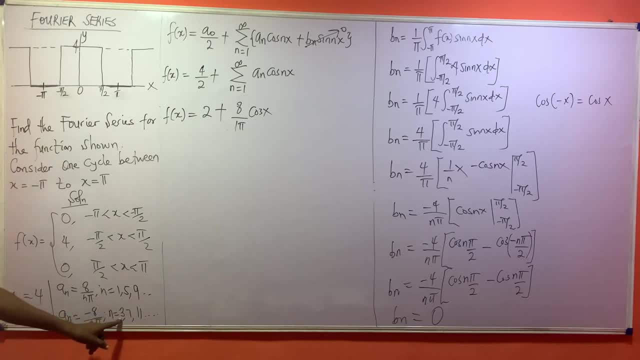 Let us go to the next one. When a sub n will be giving us 3, what's going to become our a A sub n When n is equal to 3. I'll be having minus 8 over n pi. This is minus 8 over n pi. 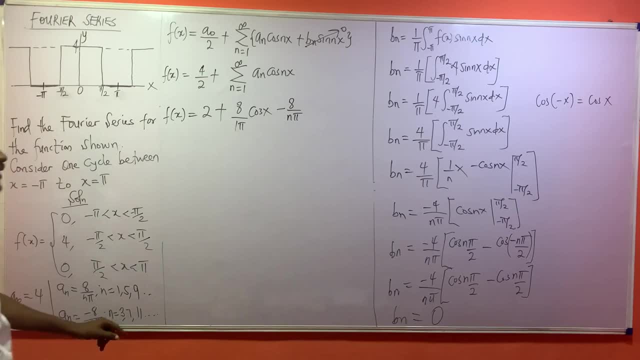 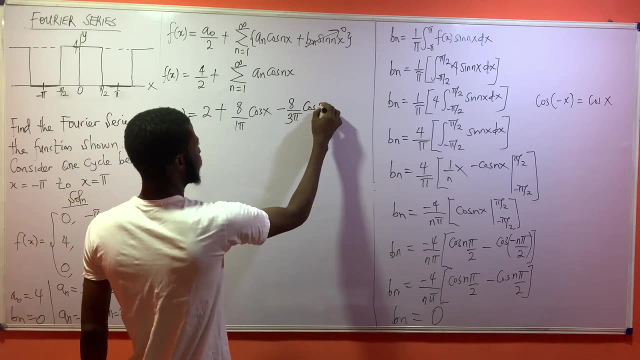 But remember what am I talking about? The third, when n is equal to 3. So this n here should become what 3.. So n should become what 3. Then I'll be having cos 3: what? 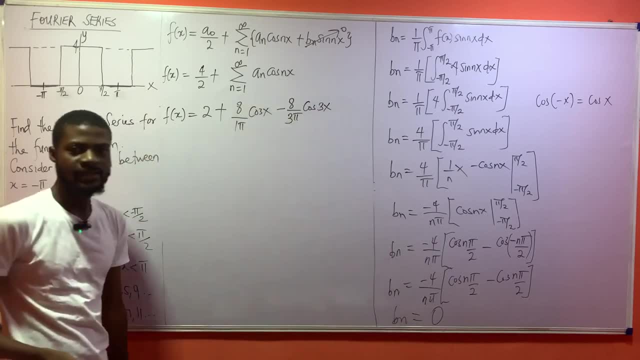 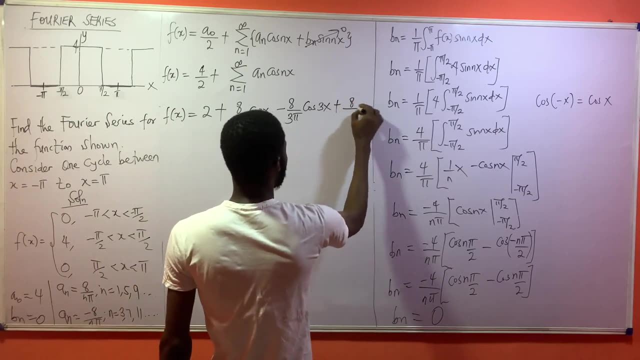 x, 3x, because my n is now 3, right, Okay, I go to the next one, 5.. Go to the next one, 5.. So this is plus 8 over n pi. But what is my n? 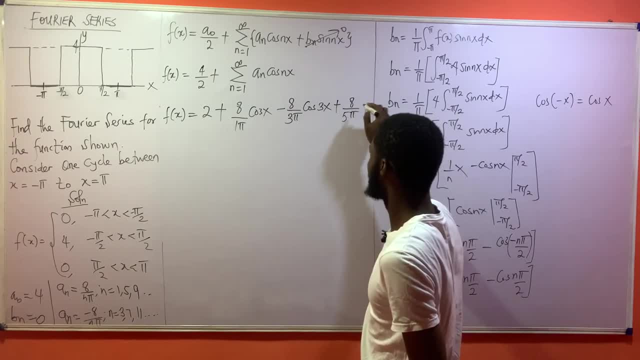 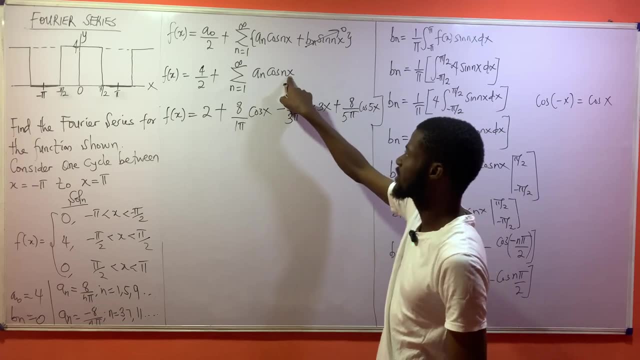 n is what 5.. So I can remove this, my n, and put 5. And this will become cos what 5x. It will become 5x because we have nx. So our n is what. 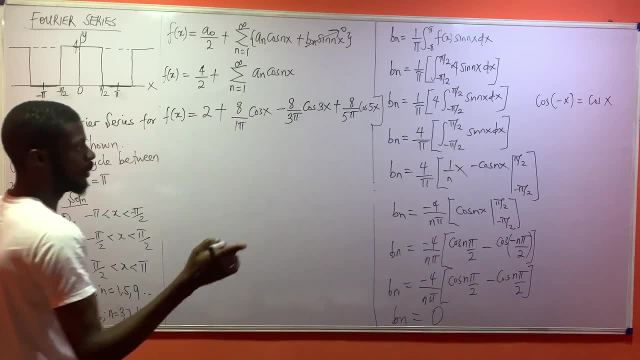 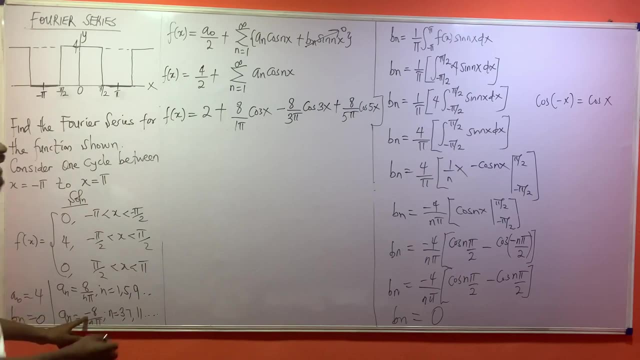 5. The next one: again, I'll just add one more. I'll just add one more because we cannot really add an infinite amount. It's not that madness, So you can't really do that. So the next guy will then become: 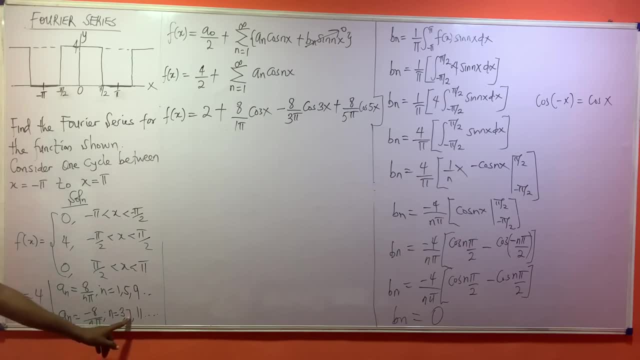 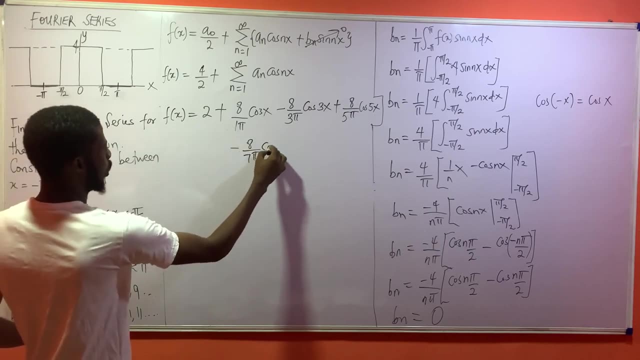 This is 5, right, So I'll be talking about 7 this time 7.. So this will become minus 8 over 7 pi cos 7x, Then plus. I'll just do all of those continuously. 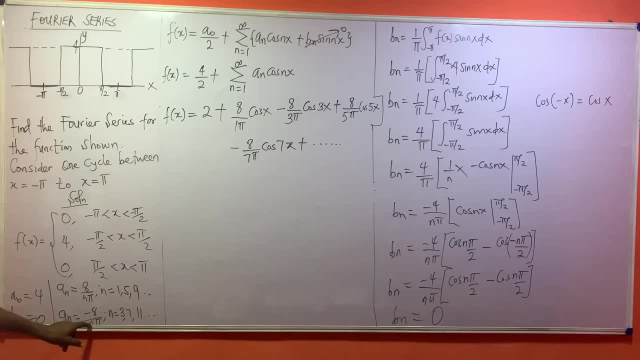 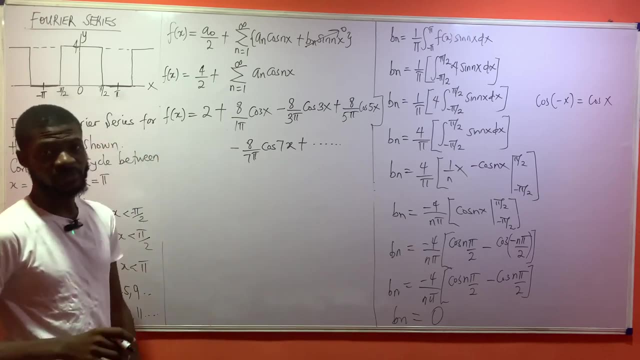 Okay, So I said 8 over 7, because my n is now what? 7.. Now can I actually factor this out in a way, Can I make it much more beautiful in a way? Now I can say that this is f of s. 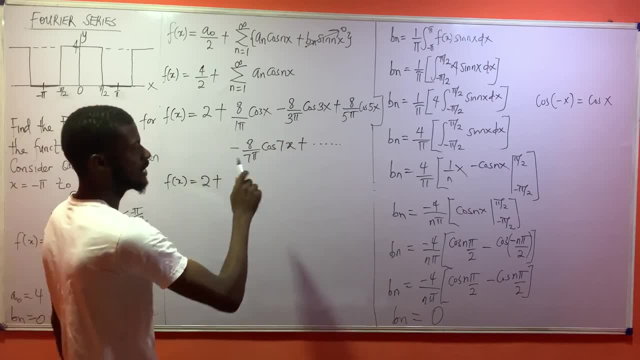 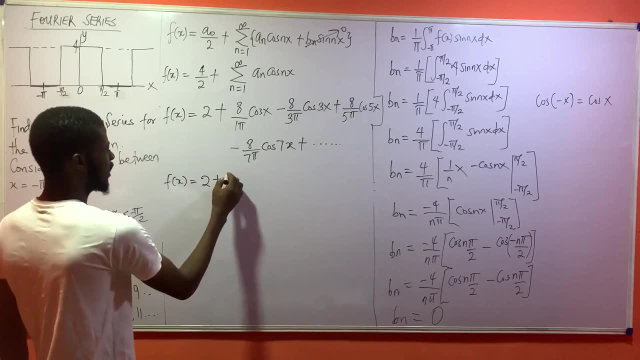 Okay, For 2 plus. If you look at every single function here, I have 8 over pi, 8 over pi, 8 over pi almost everywhere. So I can factorize it as 8 over pi. Then I open a bracket. 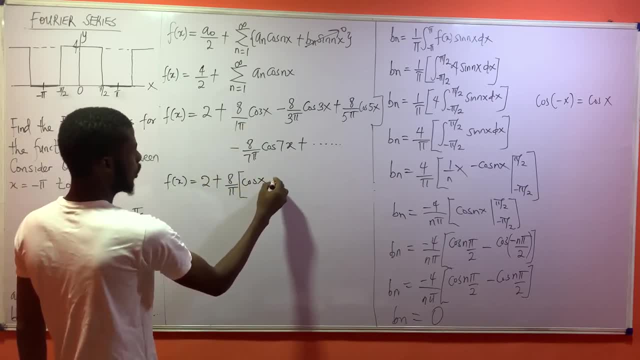 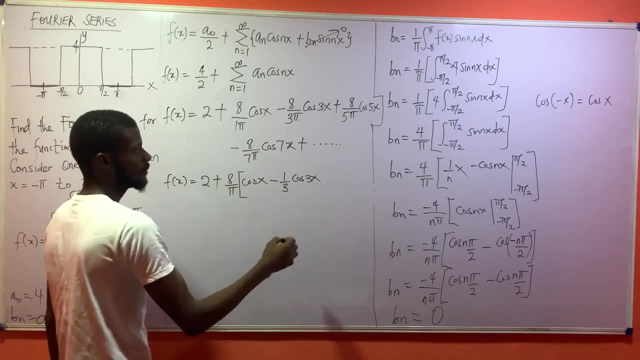 If 8 over pi leaves what will be remaining? Cos x, Then minus 8 over pi leaves what will be remaining. 1 over 3 cos 3s will be remaining. Plus 8 over pi leaves what will be remaining. 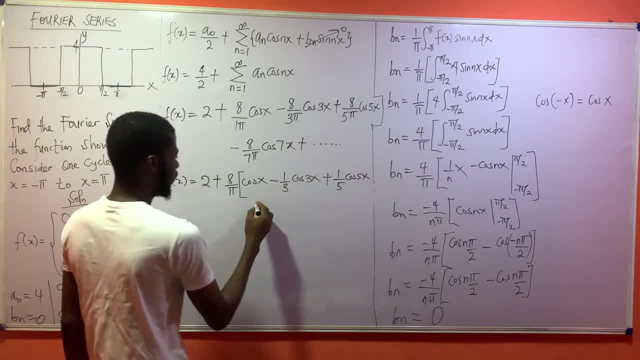 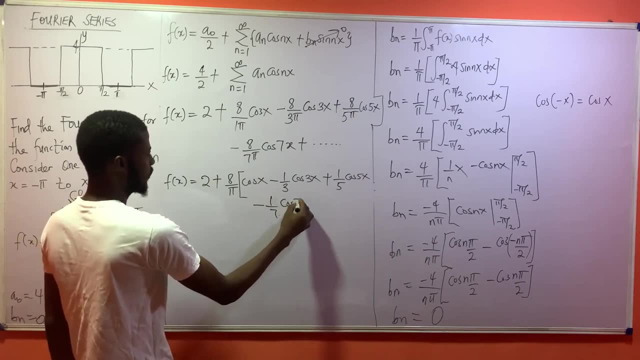 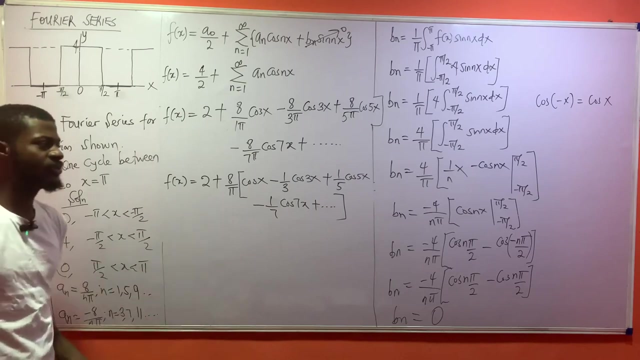 1 over 5. Cos 5s. Then minus 8 over pi leaves what will be remaining 1 over 7. Cos 7x: Then you add all those guys. So this is going to become what the Fourier series is going to look like. 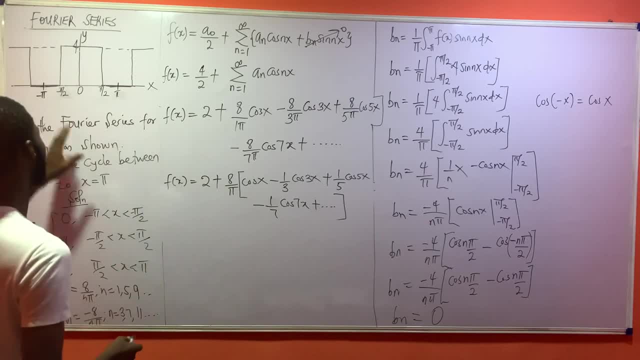 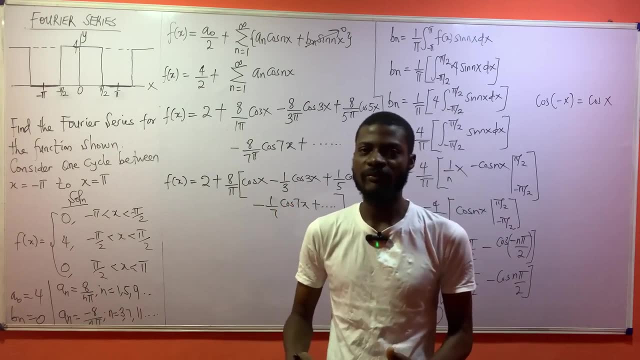 So this will become the final answer for this very guy. So very soon, in my videos, I'm going to be displaying all of this thing with a graphic calculator to display, So I'm going to be showing you how to do this very infinite amount.